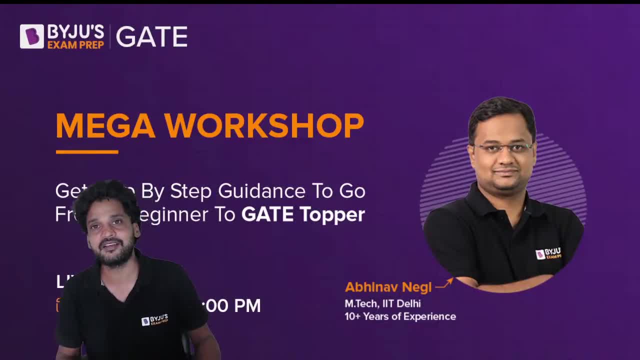 There's only one definition for that: If you are in between 0 to 100 rank, rather 100 to 0 rank, you will be considered as a topper. But anyhow, you will be given all the tips and tricks to crack the GATE exam with the best rank. So if you are aspiring for the GATE, no matter which year you are eyeing for, you will be given the complete details, the complete idea. You will be directed and you will be guided properly in this very session. Please do not miss this session, which is coming live on your way on the 19th of November 8pm. 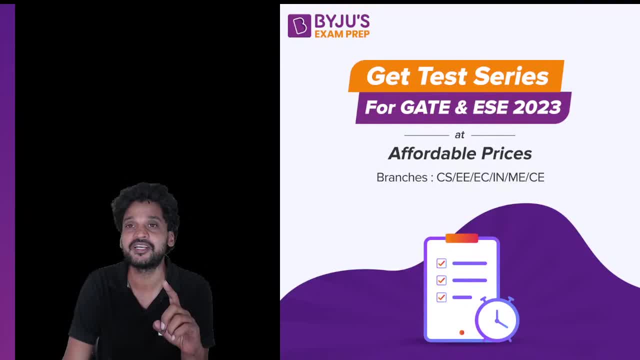 And please download the test series. I request you people to download the test series, which is available at the very affordable prices, because this is the right time for the test series, needless to tell you people, Because here, right now, we people are in, you know, at the end of the November till November to the January, we have only one limited time, a very limited capsule of the time, in which we just have 60 to 70 odd days. This must be predictively and potentially utilized by attempting as many test series as possible. 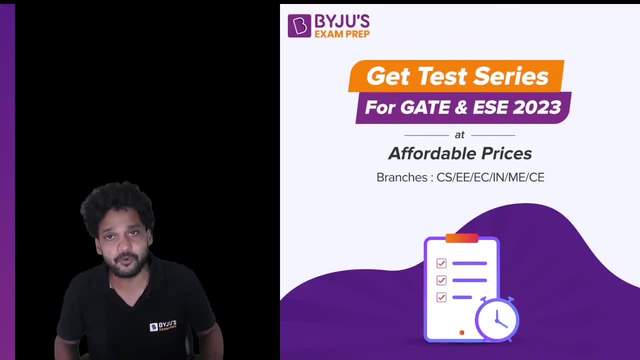 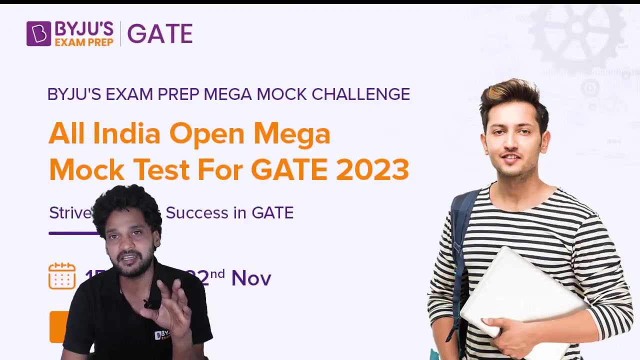 So you know, by just example, we are providing you as an initiative to help your students out. the test series are very, very affordable prices. So make use this, make most out of this, Excuse me, Make the most out of the test series and just hi, Anu, very good evening. And then just you can, you'll be able to, you know, crack the GATE exam very, very easily, because the test series let me tell you, which is going to give you a different dimension for cracking the GATE exam. 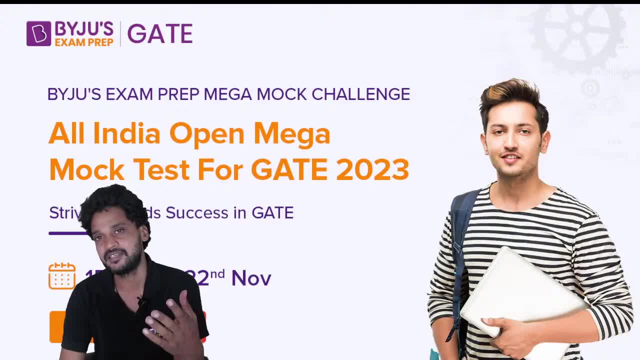 Because the GATE exam you will be familiar with. The moment you attempt the test series, you will get to know what all the type of questions that you're going to get. Now, one more important thing is this: This is the time for the mock test, right? 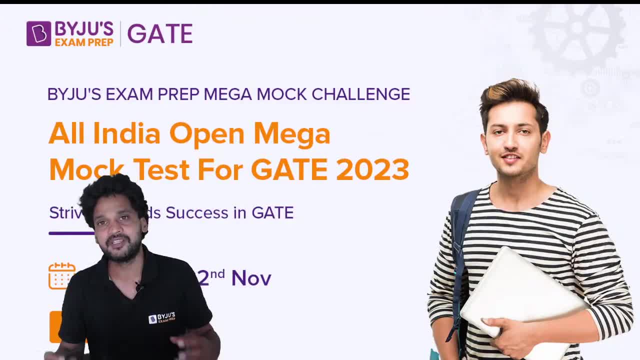 The mock test will give you the idea, the basic idea, the. you know the blueprint of the PAPO pattern. So it is also the time for the mock test. The mock test is coming live in your way from the 15th of November to 22nd of November. 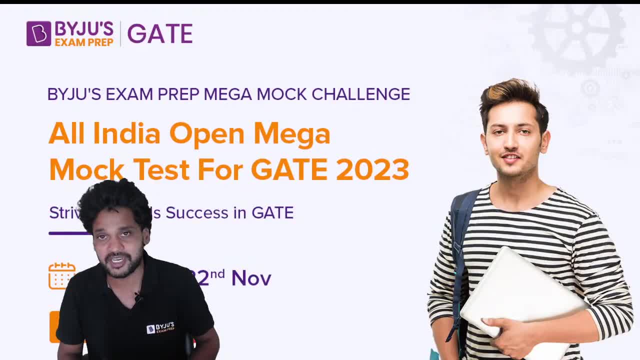 The mock test will be live. You just give the mock test And first of all, you just need to get registered. If you haven't already yet, do get registered to the mock test and give the mock test, And you will have to wait for the result. 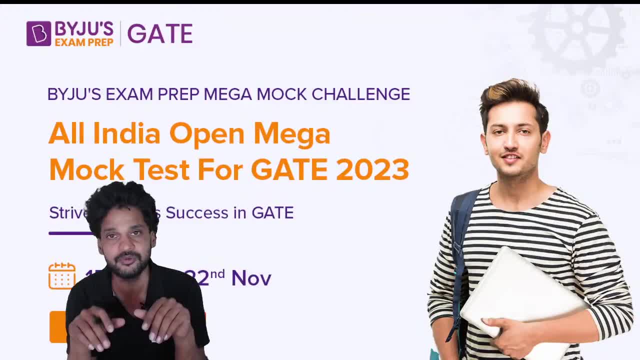 It is going to be announced on 23rd of November, 3rd of this month, So these two are mandatory things. First of all, get the test series. Second thing is, do not miss the mock test at all. So let me take you people. 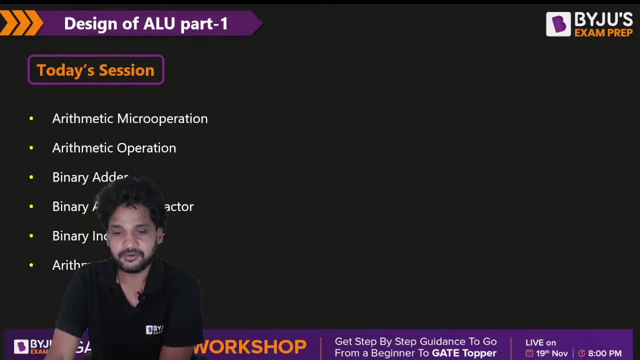 Download the app. Yeah, Now the today's session. Excuse me, I am going to move this side. It is behind me, I guess. Yeah, but anyhow, I am going to discuss about the arithmetic and logic unit. In the arithmetic and logic unit, 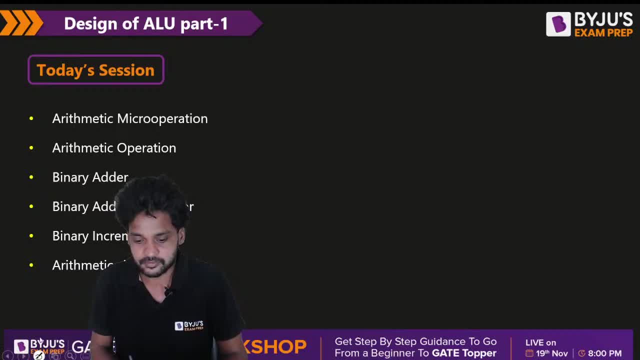 let me tell you, In the arithmetic and logic unit, let me tell you, There are three different components. The first one is arithmetic unit, Second one is logic unit And the third one is 50 unit. Okay, These three units will be clubbed together. 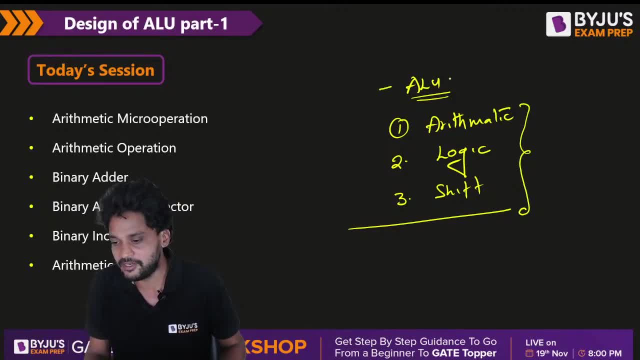 Because, when you talk about ALU, ALU is able to perform a wide variety of operations. The first type of the operation that can be performed by any ALU is the arithmetic operations. What are the basic arithmetic operations that can be performed by the ALU? 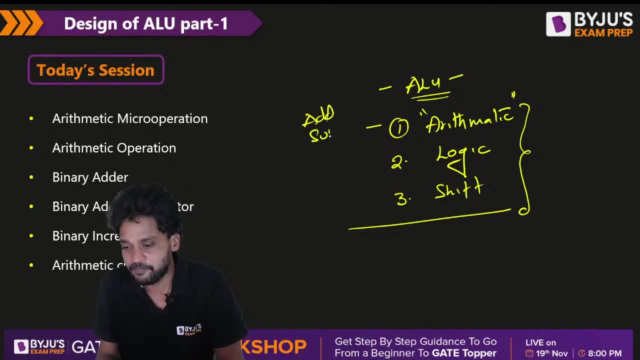 ALU is able to perform addition, subtraction, incrementing and decrementing. ALU is also able to perform the logic operations. Logic operations are and are not There are. altogether, we do have 16 different logical operations, including set and clear What is set. 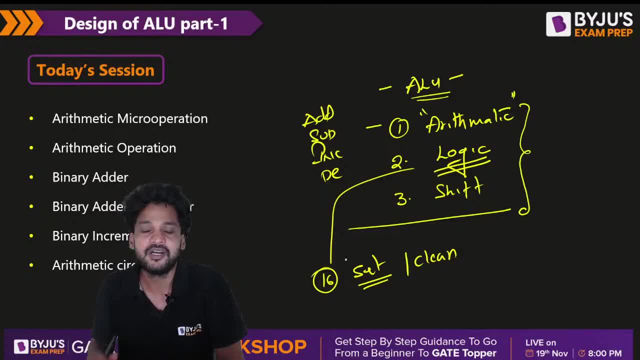 If you perform set operation on any register, all the digits of the register will be set. If you perform clear operation on any register, all the digits of a register will be cleared. That is the difference between set and clear. Okay, So finally, shift operation. 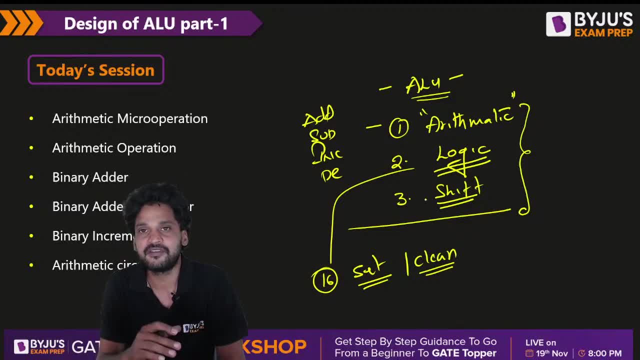 What is the shift operation? There will be right shift. there will be left shift. The contents of the register will be shifted right or will be shifted left to one bit position. when you perform this shift, It could be a right shift or the left shift. 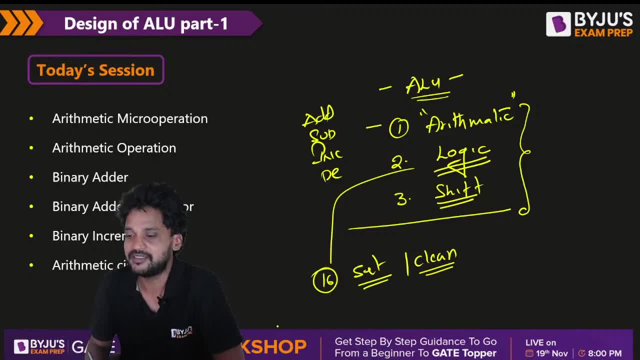 Now, when you talk about ALU, ALU is a multiplexed unit of arithmetic unit, logic unit, shift unit. All these three units will be differently designed or manufactured. Finally, all these three units will be multiplexed. This multiplexed unit. 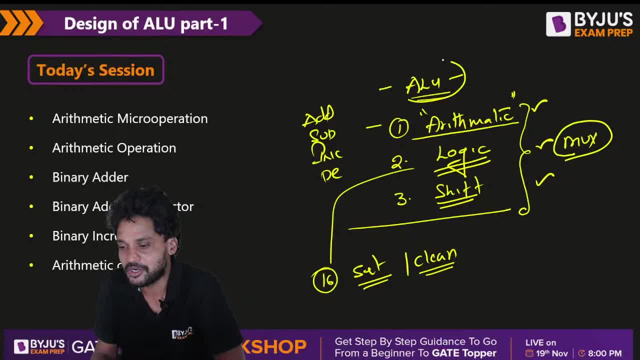 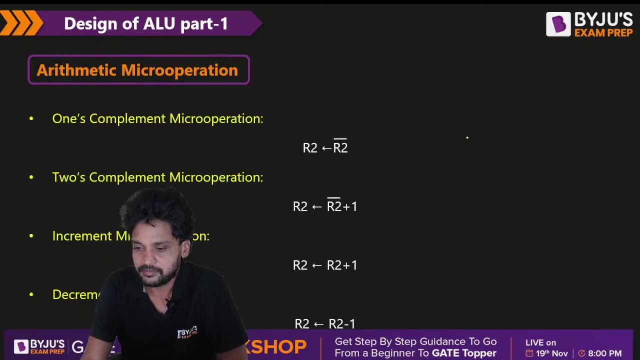 of all these three units together is called an ALU. Got me. Now we don't need to discuss about the logic unit. Let me tell you, Let me go to the next term Here: arithmetic, logic and shift unit. I need. 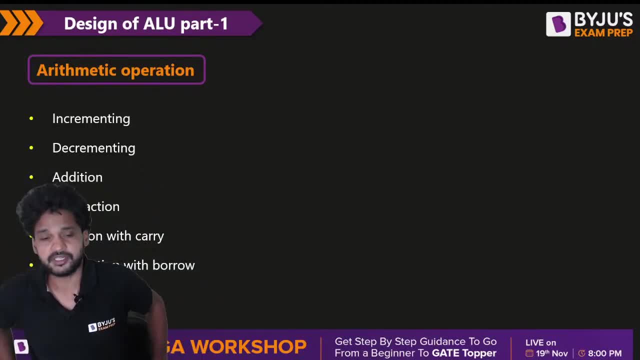 to position myself towards, I guess, the right or left. No, no, no, I think this is that way, because, Yeah, No, I think I am being cut, But anyhow, I will explain. But anyhow, I will explain. Stay focused here. 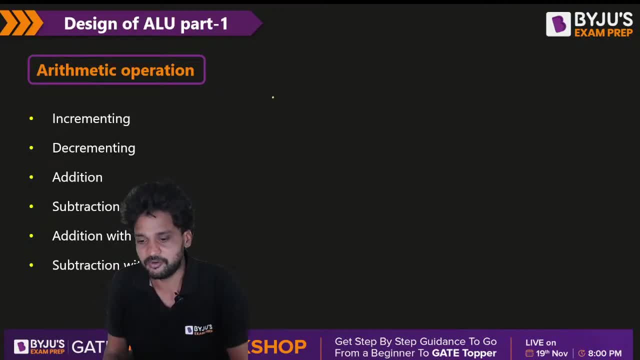 I am going to write all the arithmetic operations that are going to be performed. There are only four basic arithmetic operations that are going to be performed by the ALU. What are those? Addition. second one is subtraction and the third one is incrementing and the fourth one 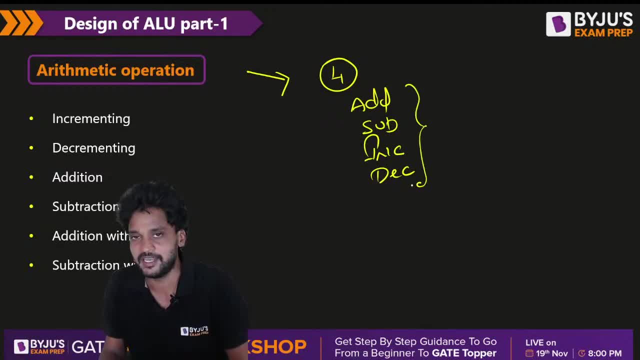 is decrementing. These are the only operations performed by the ALU, Not multiplication, not division, Because multiplication and division are the shortcuts for addition and subtraction. If you want to perform multiplication, some addition should be performed in loop. If you want to perform subtraction, some. 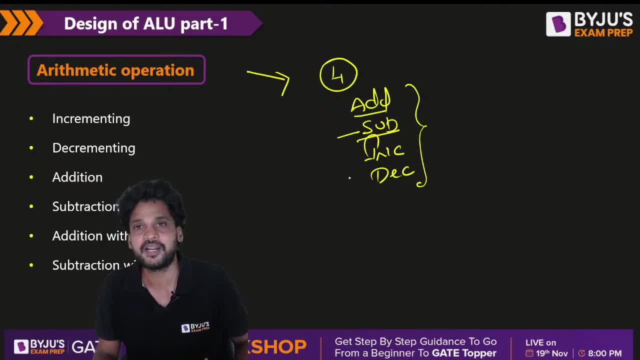 subtraction must be performed. Sorry, If you want to perform division, some subtraction must be performed in loop, And incrementing- decrementing are also the operations that are going to be carried out in an ALU And similar to that we do have. 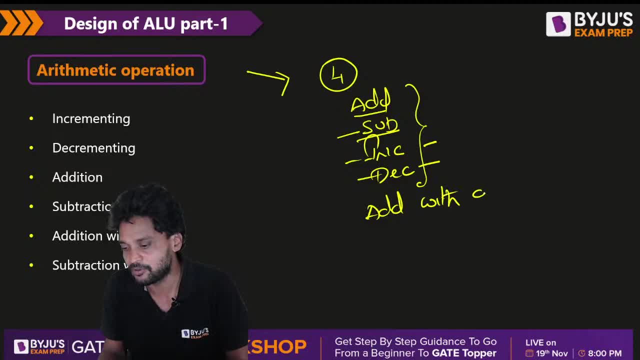 addition with carry and subtraction with borrow Okay. Subtraction with borrow Okay. These are all the operations that are going to be performed by arithmetic units of an ALU. Now what we are going to do is we are just going to. 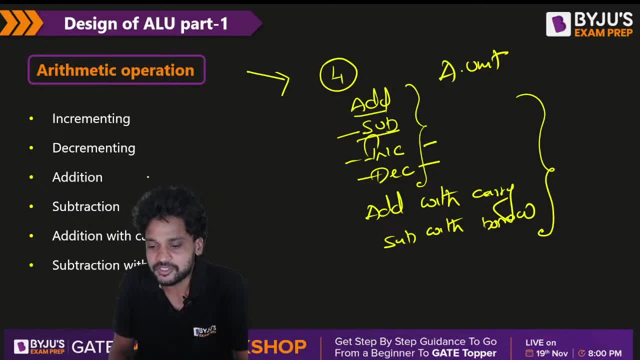 build all these units differently. Finally, we will club all the units. That means we will start with the incrementing unit and then we will go for an addition unit, followed by subtraction unit and finally we are going to design a complete unit which can perform. 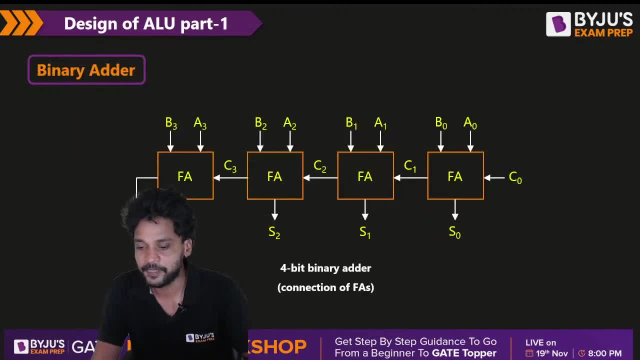 addition, subtraction, incrementing and decrementing. Now let us have a look at it. I hope it is completely visual. Okay, It is a 4-bit ADO. It is a 4-bit ADO, See my ALU. 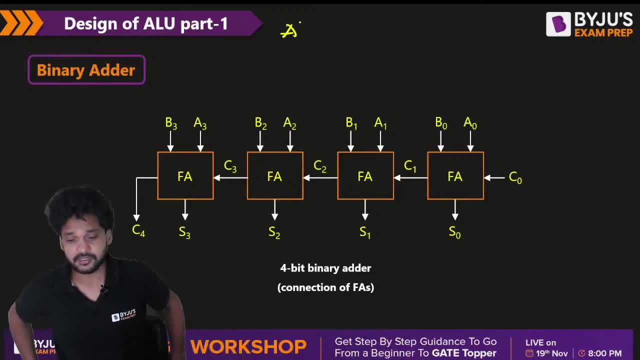 excuse me, I guess I need to come this side. This is the layout is not correct. Yeah, I hope now it is completely visual right Now. have a look at this. The thing is this is here. Stay focused. 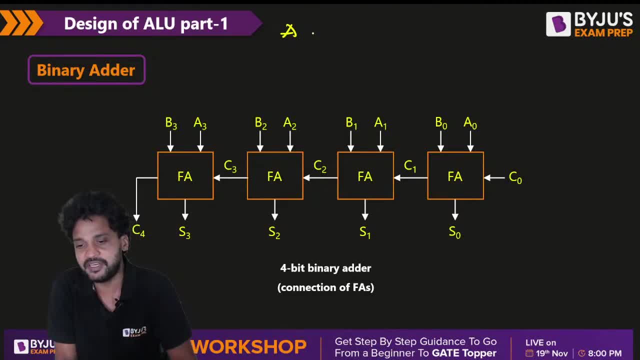 Now, when you want to perform addition, first of all, we need to define the operation. in order to design and construct any unit, The operation that is needed to be performed is an addition. What is addition- Let us say A- is the. 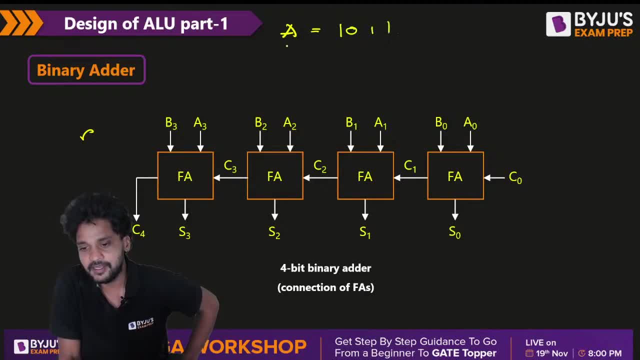 4-bit number. A is equal to, let us say, 1011.. B is another 4-digit number. B is equal to 1101.. Clear Now, these must be added In order to add a 4-digit number. what do we require? 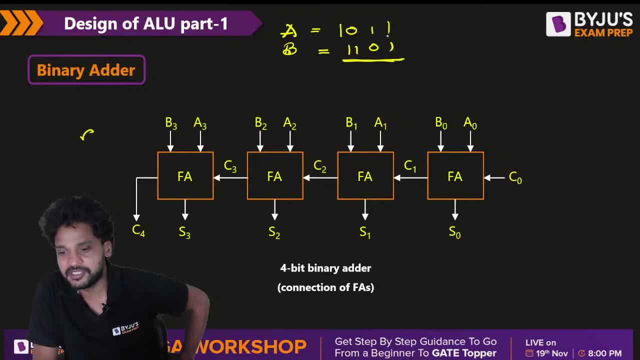 Simple, understand, Least significant 2 digits must be added. 1 plus 1 is equal to 10, right 0 here: 1 here. 1 plus 1 is equal to 10, right 10 plus 0 is equal. 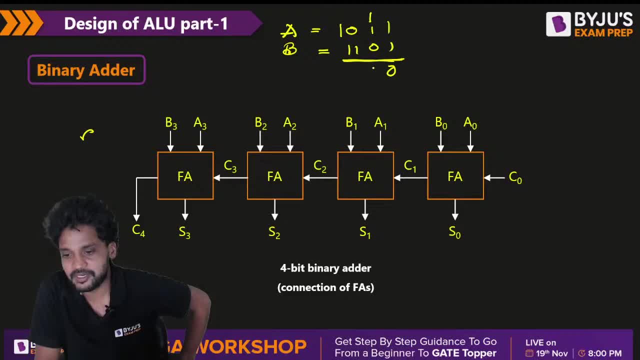 to 10.. So 1 plus 1 plus 0 is equal to 10, 0 here, 1 here, 11, 0, 1, 111, 1, 1.. So there will be an end carry And 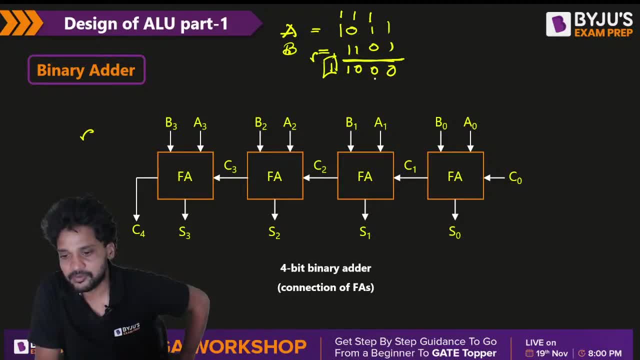 here once again: 11,, 10,, 10,, 11, 10,, 11, 10, 11, 10, and 111, 11.. So once again, yeah, Now understand carefully. 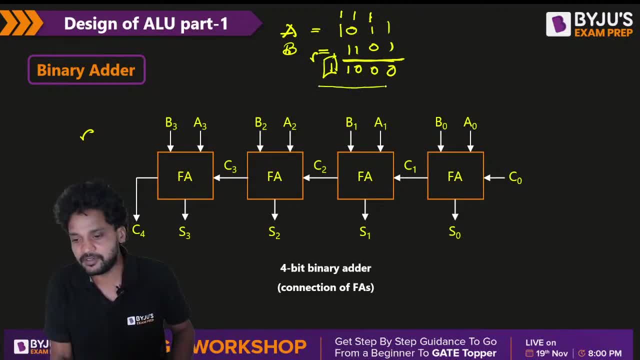 See, when you look at the operation, what is being performed Here. I am adding 4-digit number. Okay, When you perform 4-digit addition, what you require is our 4 full adders must be connected together In the 4-digit addition. 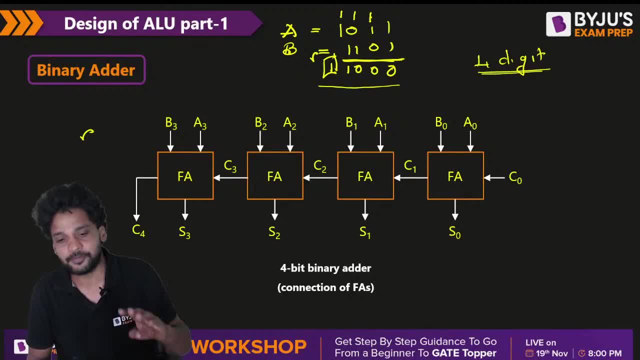 you must be able to collect 4 full adders together. Now understand, Before I take you people any further, understand this one very carefully: The ALU, any ALU, is defined by the supporting bits, For an example in: 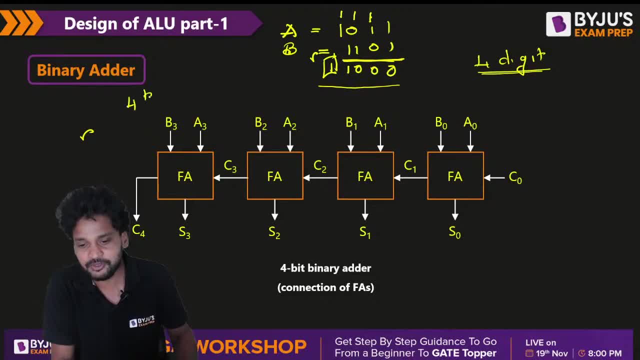 the real-time world. we have 4-bit ALUs or 8-bit ALUs. What is a 4-bit ALU? A 4-bit ALU can perform a 4-bit addition at a time. For an example, you want to perform a 16-bit. 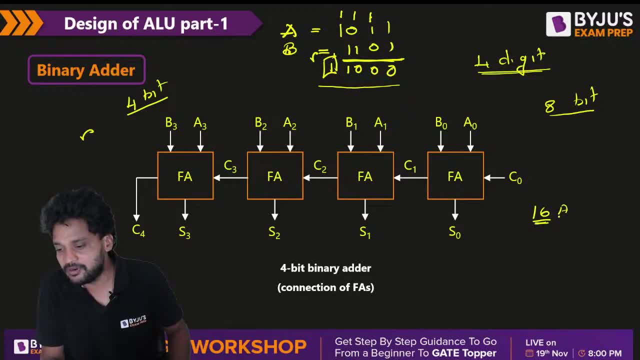 addition. So A is a 16-digit number, B also is another 16-digit number, But if it is being carried out in a 4-bit ALU, all these total 16-digits will be divided into 4,, 4,, 4,, 4.. 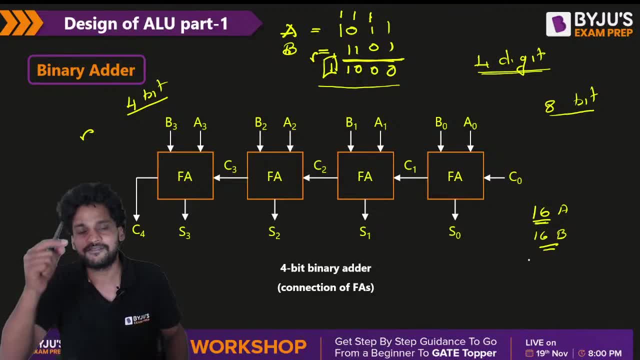 Least significant 4-digits will be added to B in the first phase and next 4-digits will be added in the second phase. next 4-digits will be added in the third phase. next 4-digits will be added in the. 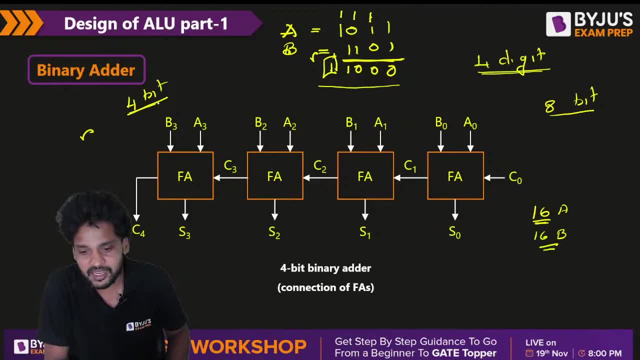 fourth phase. So by using a 4-bit ALU, if you want to perform a 16-bit addition, that will get carried out in 4 phases. Least significant 4-digits, next 4-digits, next 4-digits. 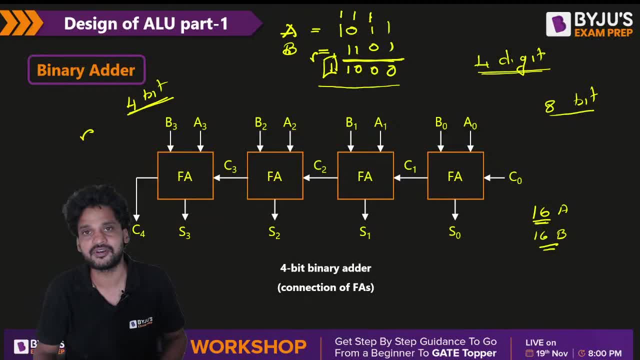 and next 4-digits. What we are witnessing right now on the screen is a 4-bit ALU and a 4-bit ADO. Now let us have a look at. in this, what we are going to do is least significant 2-digits. 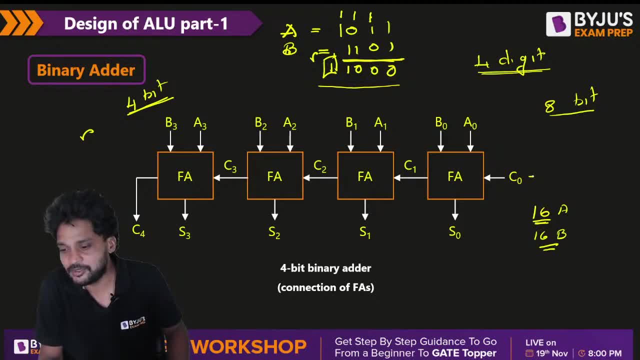 will be applied to the first full ADO And carry 0,. I mean C0 will definitely be equal to 0.. ALU can perform operation on 4-bit data at a time. Our ALU if it is an 8-bit ALU. 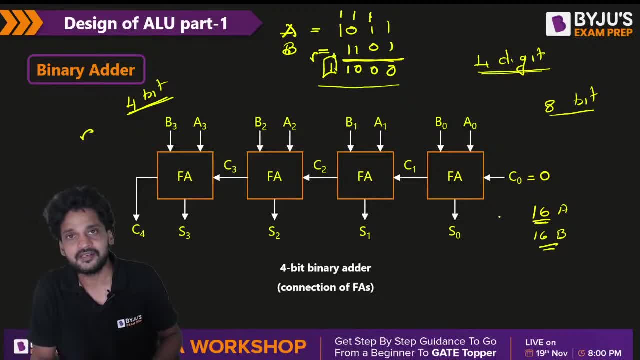 8-bit. ALU can perform addition on 8-bits at a time, But now we are discussing only 4-bit. in order to make the things very simple Now let us say this is an intermediate stage, Because there will be total 4 stages. 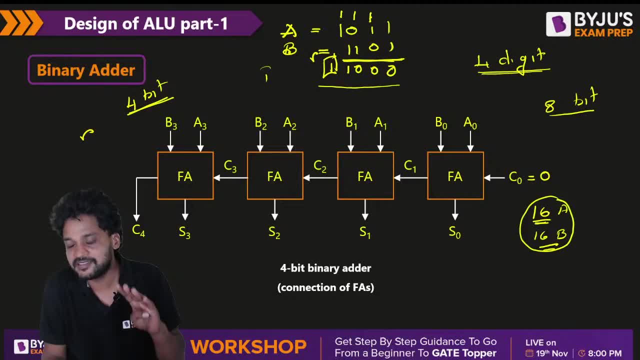 Let us say we are performing a 16-bit addition. This 16-bit addition must be performed in 4 stages. Now understand if it is an intermediate stage- intermediate stage- this C0 will be collected from the previous stage. C4 will be connected to the. 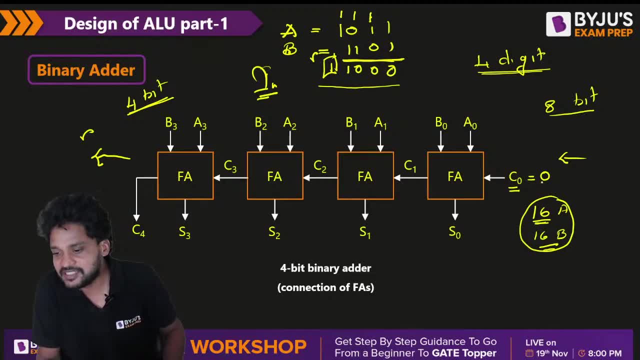 next stage. If it is the first stage, C0 will be 0.. If it is the final stage, the produced C4 is the end carry. Okay, So understand this. Anyhow, we are not performing 16-bit addition. 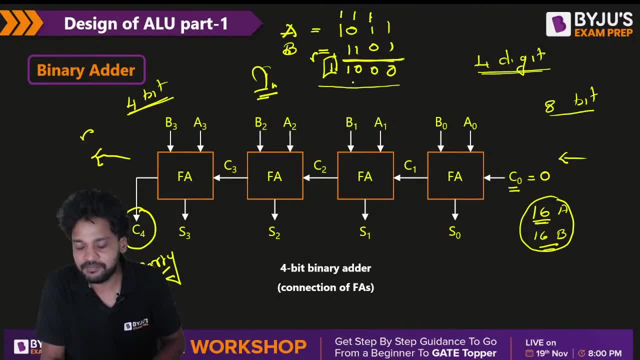 Let us, in order to keep the things simple, let us keep the discussion only for adding 4-digits Initially, A will be equal to 1.. Rather, you know, these 2-digits will be applied here. These 2-digits will be applied here. 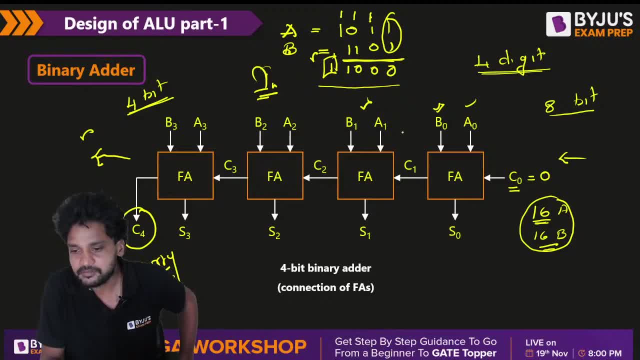 These 3-digits Excuse me From the next section. we got A1 and B1. And this carry will be given here. Similarly, these 2-digits will be applied here. The carry will be given here. 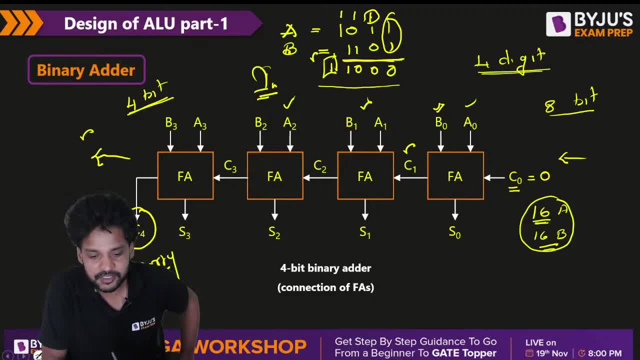 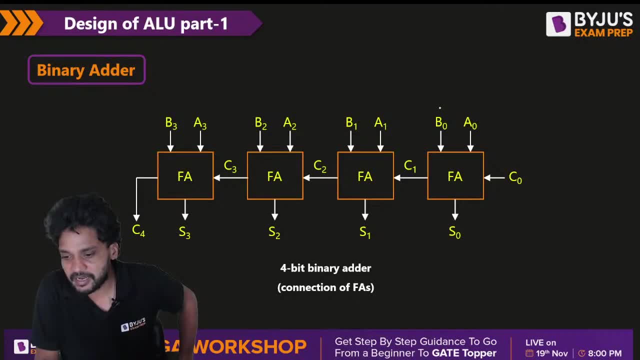 And finally, A3 and B3 will be connected here. So let me clear this and explain you for one more time. So A0 and B0.. The least significant 2-digits will be applied here, So A0 will be equal to 0. 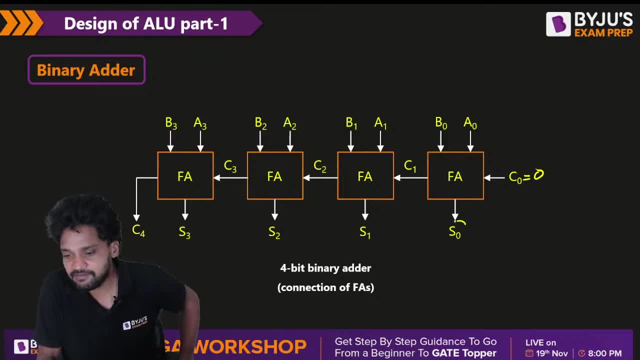 These 2-digits will be added. Some will be produced here. Carry will be given to the next stage, So this full addo will perform an addition in between carry 1, A1 and B1.. All 3 together will get added. 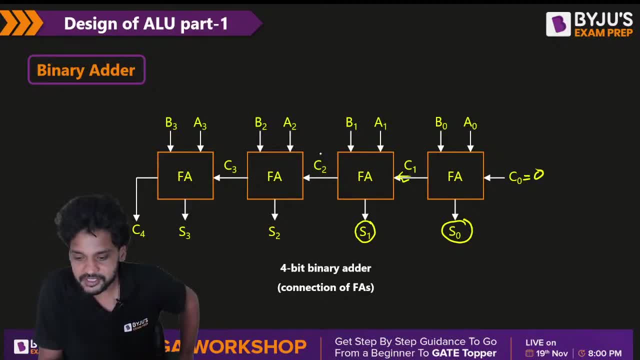 And some 1 will get produced here. You know the carry 2 will be given to the next stage of the full addo. So in the next full addo C2, A2, B2 will get added. 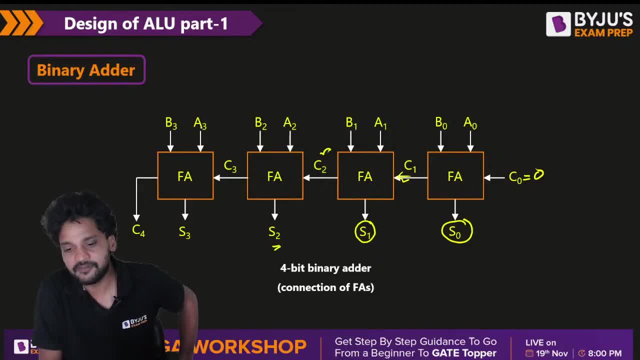 Some will be here. Carry will be here. In the next full addo, of course, A3, B3 and C3 will get added, And some will be produced here. Carry will be produced here. This is what the addition is all about. 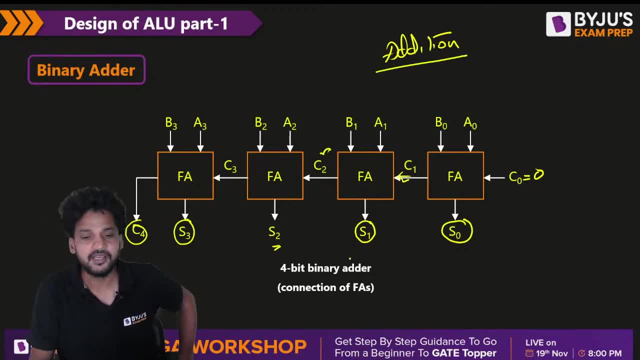 This is what the addition is all about. So this circuit is an adder circuit. This circuit can simply perform only addition. But what if we want to correct 4 parts of operation, 3 inputs and carry outputs? Exactly what you told is right. 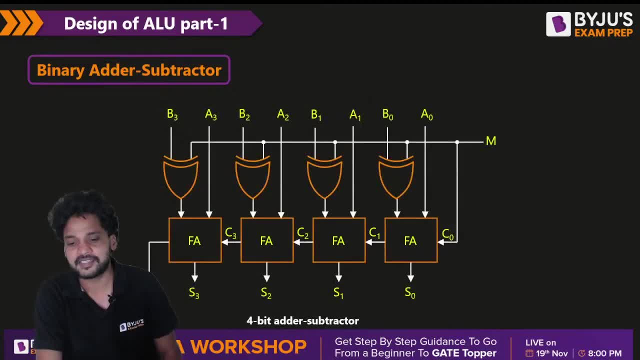 or wrong. Next thing is: we are going to discuss about adder-subtractor unit. We are going to discuss about adder-subtractor unit, How adder-subtractor unit is going to be designed and discussed in this time. See in the adder-subtractor unit. 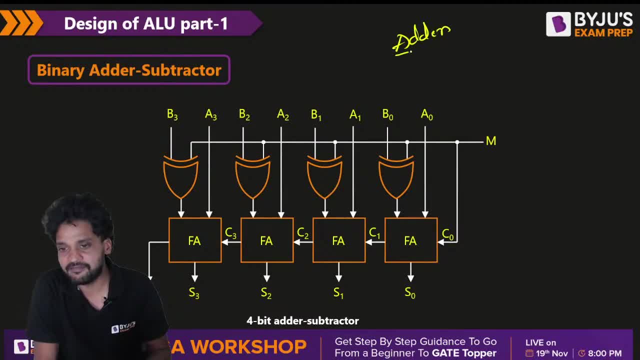 of course, this unit is similar to the addition unit, adder unit, only, Only with one slightest difference. What is the slightest difference? Let us have a look at All the full adders: first input is equal to A. All the full adders: first input is equal to A. 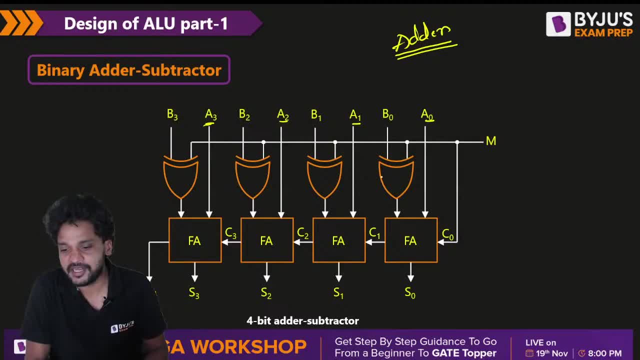 Second input, if you can have a look at, B is not directly connected to the full adder. B is connected to the full adder via an XR gate. There are 4 XR gates. To the XR gate B is connected. 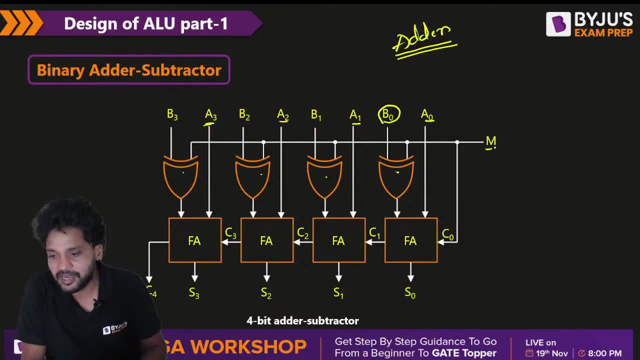 XR gate's. second input is taken from a line M. Just once again have a look at. There are 4 full adders. Full adders require 3 inputs. One input is from A, One more input is from the digit M. 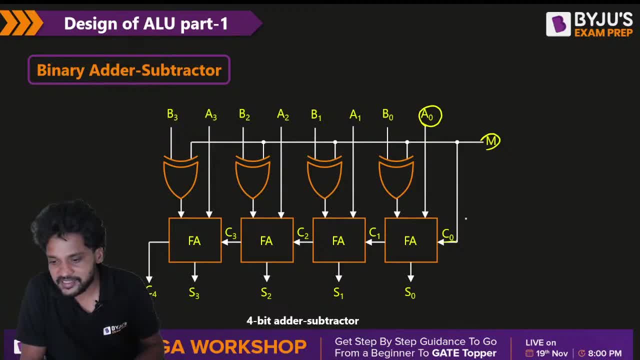 This is the carry in right. Carry is actually taken from a digit called M. Now the third input of the full adder, just have a look at: One input is A, one more is carry. in The third input which has to be collected from B: 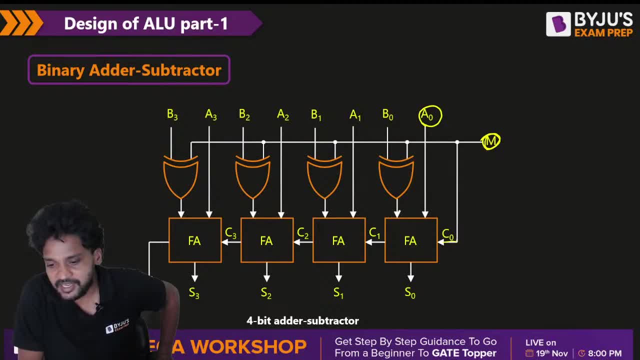 has actually been taken from an XR gate. We of course this is A, This must be from B, right, But we did not connect it directly. Rather, B is connected to an XR gate. The output of the XR gate is connected to the full adder. 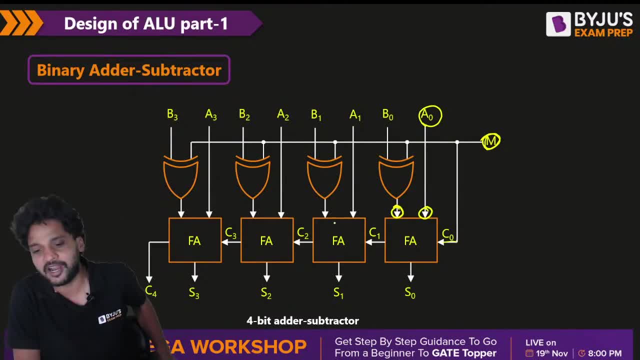 Here also. B1 is connected to the XR gate. Output of the XR gate is connected to the full adder. B2 is connected to the XR gate. Output of the XR gate is connected to the full adder. B3 is connected to the XR gate. 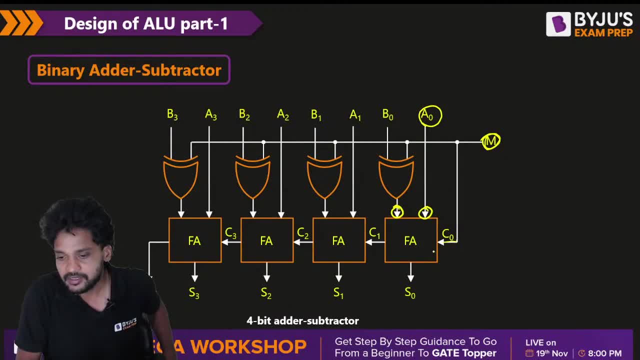 Output of the XR gate is connected to the full adder. Now, how the circuit will be able to perform addition, How the circuit will be able to perform the subtraction. For that understand, the XR gate's second input is taken from the bit M. 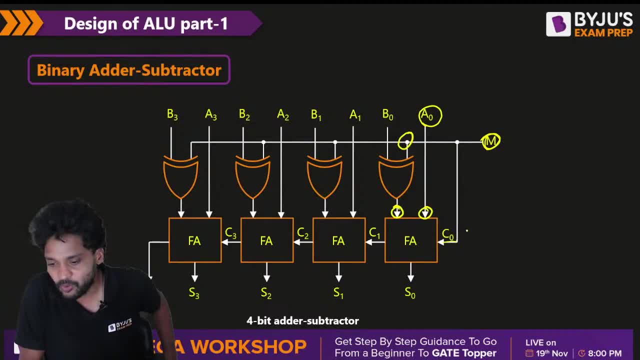 Yes or no? The M is providing two inputs. One is carry, One more is second input of the XR gate. In this slide, let me explain you one simple rule. When M is equal to 0, circuit will be able to perform addition. 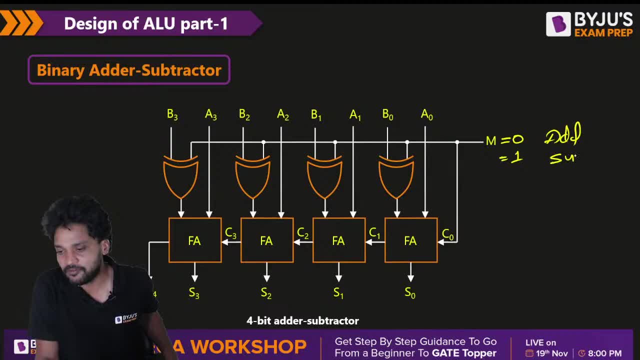 When M is equal to 1, circuit will be able to perform subtraction. Clear Why Simple. When you perform A plus B, what is needed to be performed? Simple: Full adder must add A and XR gate output must only be B. 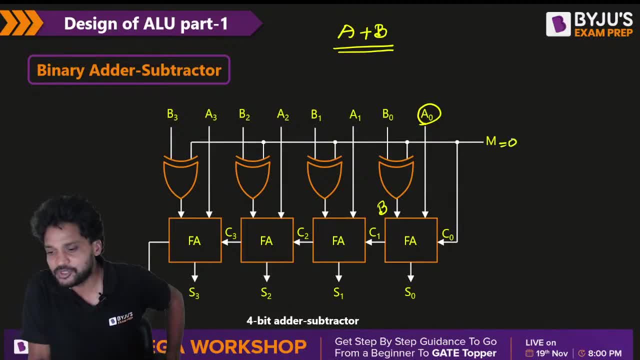 So simple. Whenever M is equal to 0,, one input of the XR gate is equal to 0.. When one input of the XR gate is 0, the output will be the other input's value. only Let us have a truth table. 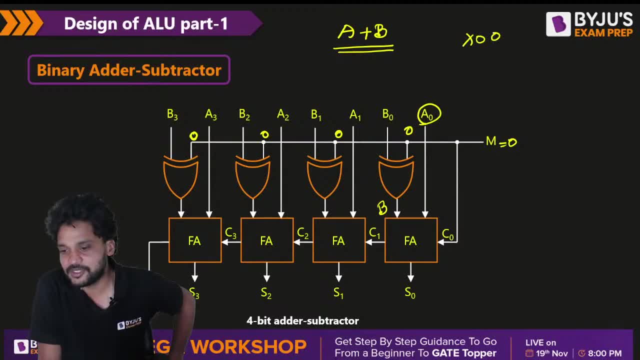 of XR gate. XR gate truth table. if you can have a look at: 0, 0, 0, 0, 1, 1. So whenever one input of the XR gate is equal to 0, the output is the other input only. 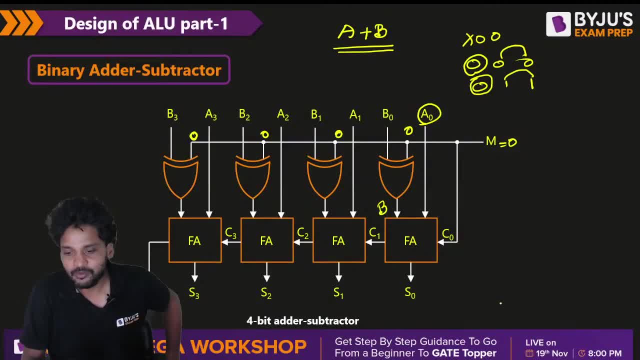 The other input will be produced as an output. In this rule. what will happen whenever M is equal to 0, XR gate will give the output from the B digit only. What will happen at that time? The full adder is receiving one input. 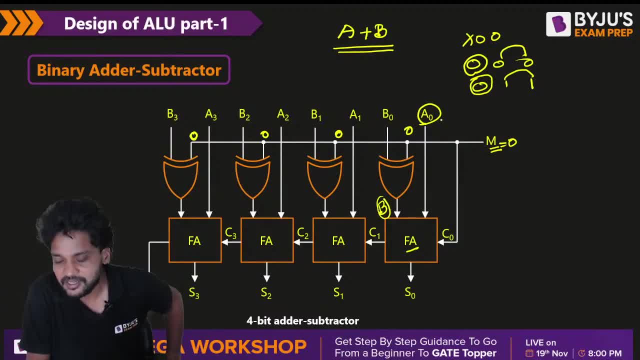 from A. One more input is from the XR, which is equal to B. So A plus B is being performed Now, whenever M is equal to 1, what is going to happen? Whenever M is equal to 1, the circuit is going to perform. 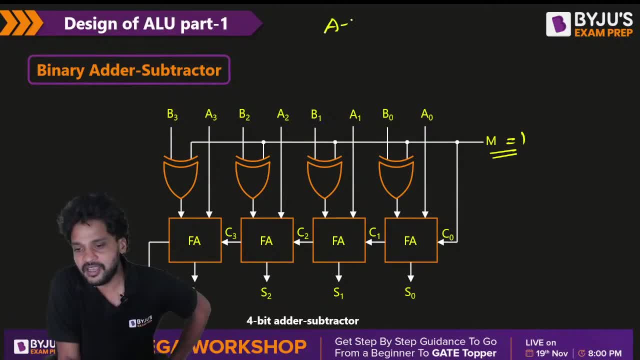 subtraction operation. Why? Let us have a look at how A minus B is going to be performed. A minus B is equal to A plus 2's complement of B. This is 2's complement of B. Now, what is 2's complement of B? 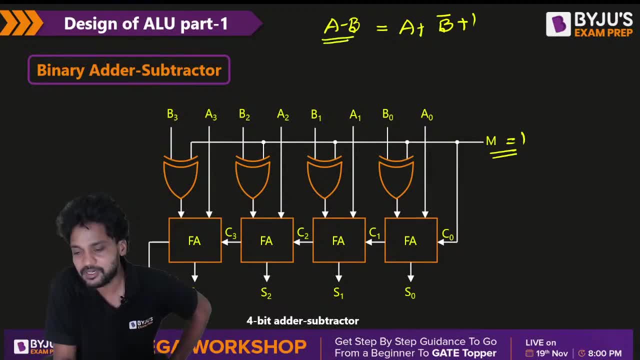 B is 1's complement plus 1.. So A minus B is equal to A plus B's complement plus 1.. This is the rule of the subtraction. So in this slide, understand, whenever M is equal to 1, what exactly is going to happen. 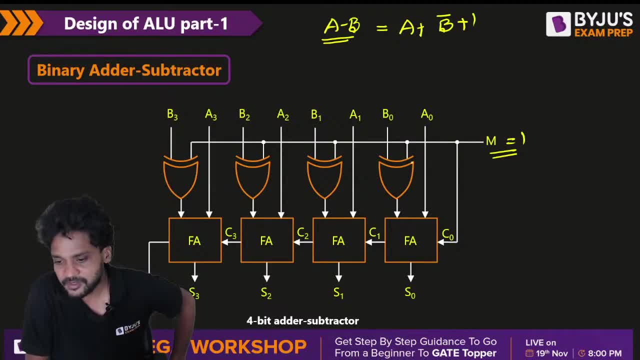 Anyhow, we are not touching A, Only B will get altered. One input of the XR gate will be equal to 1.. Whenever one input of the XR gate is set to 1, output is other input's complement. Once again, let us have: 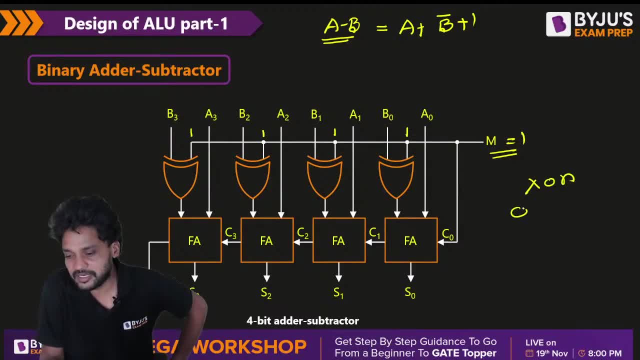 the truth table of the XR gate. XR gate truth table: 0 0 0 0 1 1 1 0. 1 1 1 0. Look at the last two digits, last two values. Whenever one input of the 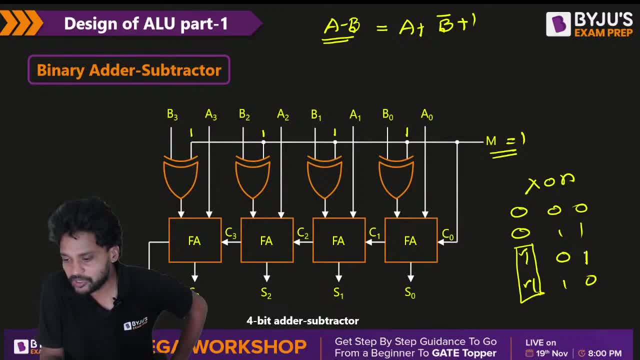 XR gate is 1, is set to be 1,. the output is next input's complement. Got me So 1 0, 1,. what is 1? 0's complement? 1 1 0. What is 0? 1's complement. 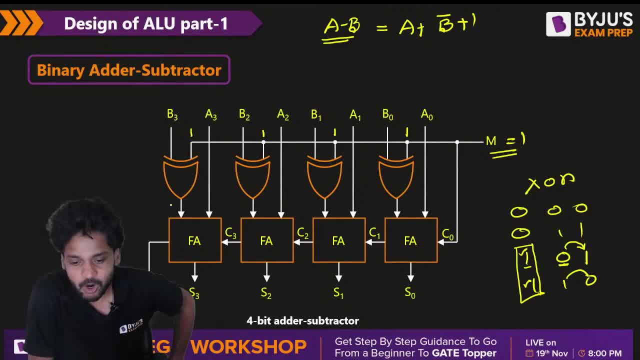 So whenever one input of the XR gate is equal to 1, output is other input's complement. Got me Complement only, not 0. So at that case, what is going to happen? Our circuit is going to perform. 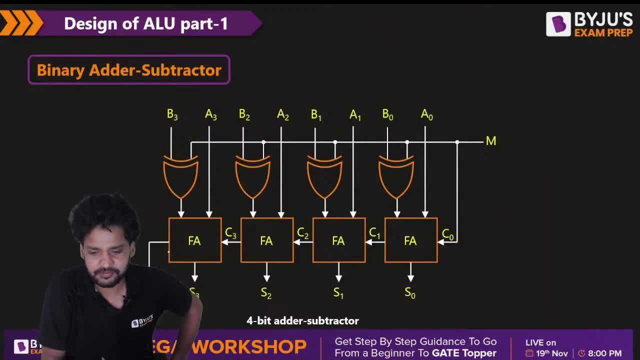 excuse me, Our circuit is going to perform A plus B complement. I said no, this is A, as one input of the XR gate is equal to 1.. All XR gates will give you B complement. Okay. And as M is equal to 1, it also makes C0 equal to 1.. 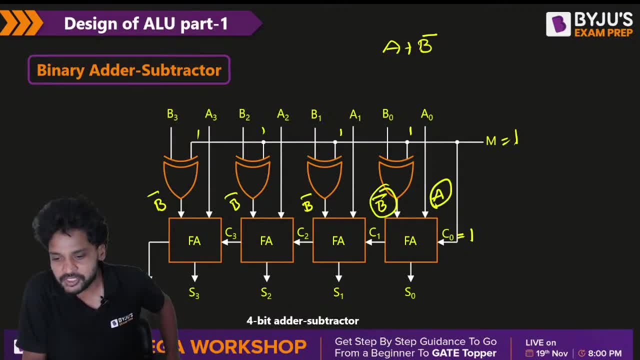 What exactly is getting performed? A plus B's complement plus 1.. So A minus B is equal to A plus B's complement plus 1, exactly is operation of A minus B. So whenever M is equal to 1, this circuit is going to perform. 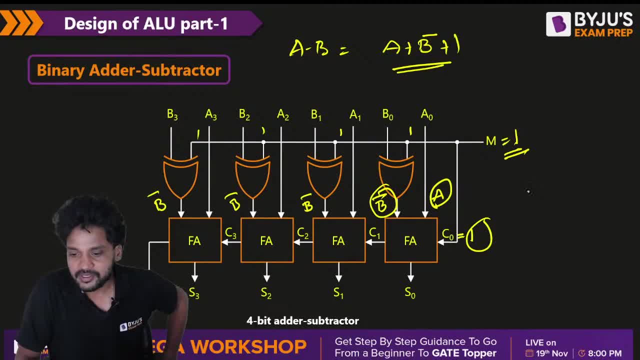 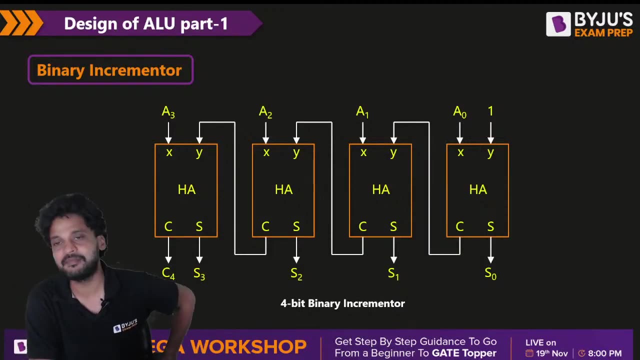 subtraction. So same circuit is performing two operations: 0 addition, 1 subtraction. Okay Next, Excuse me. I already explained this. Increment is simple. What is incrementing? Incrementing can be done very simply by adding 4 half adders together. 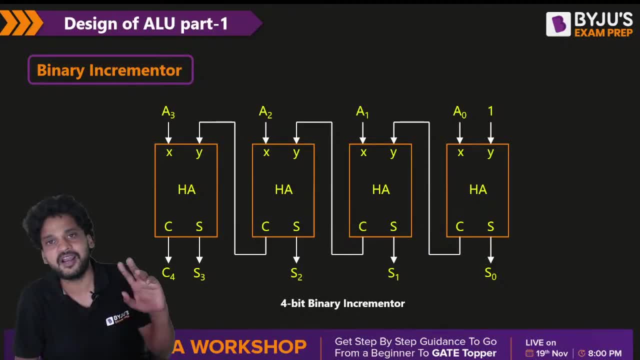 In order to simply perform incrementing, I don't require full adder. I require only half adder, Yes or no? Why? Because let us have a look at- A is equal to, let us say, 1, 0, 1, 1.. In. 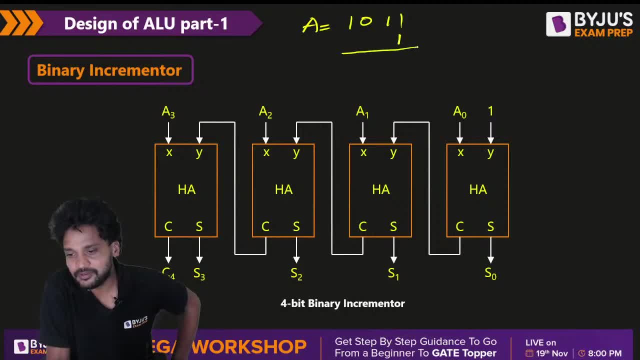 during the incrementing, we will add 1 to the total value. What is going to happen? 1 1, 0, 1. 1 here. 0 here. 1, 1. 0 here. 1 here. 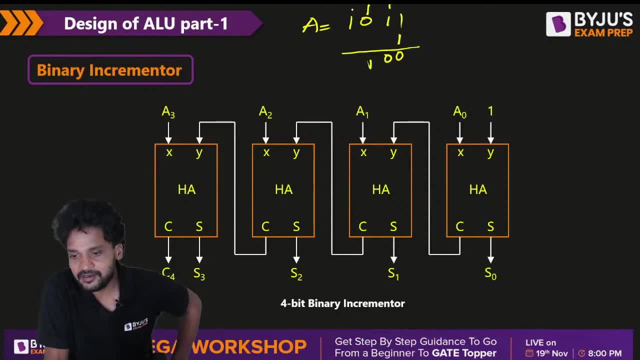 Clear: 1, 0, 1 and 0 is the carry 0, 1, 1.. At any point of period we are just only adding 2 digits. 2 digits addition. Once again, understand: During the addition, at every bit. 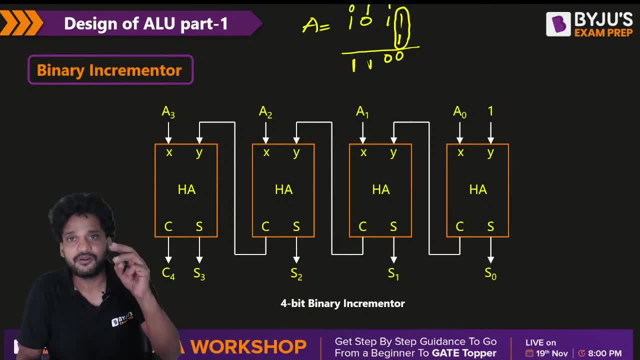 we are required to add every. in addition, we are required to add 3 digits: 1 is from A, 1 more is from B, 1 more is from carry. But during the increment we will only have 1 operand digit. 2nd digit. 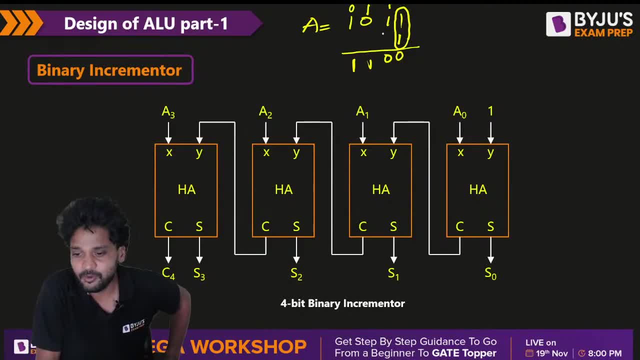 will always be carry Got me. So during an increment we require add at any at any point, only two digits. for two digit addition we don't require a full adder, we just require a half adder only. so again, in a four bit ALU it will be able to perform only a four bit. 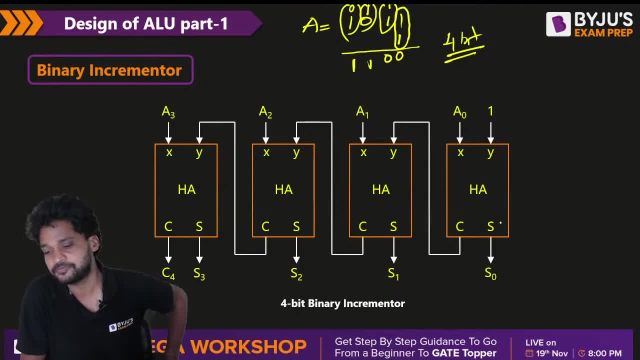 incrementing. for that i require to connect four half adders together. so simple. the mechanism is very simple. there are two inputs: x and y. x input is always from a, a0, a1, a2, a3. one input of the half adder will always be a second input of the half adder, second input of the first half adder. that is the. 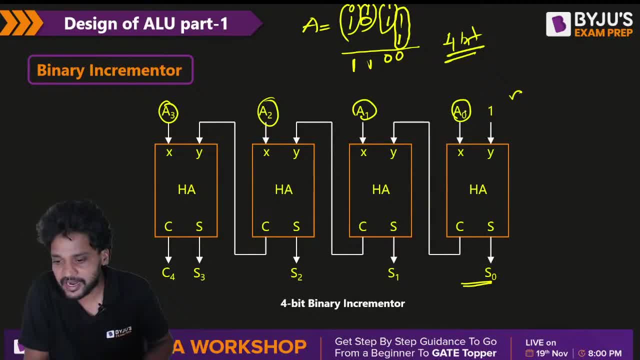 least half adder will be equal to one, because one is going to be added to a0. so here a0 plus 1 is going to produce a sum and there is a carry. the carry will be the second input of the second half adder, because every half adder requires two. 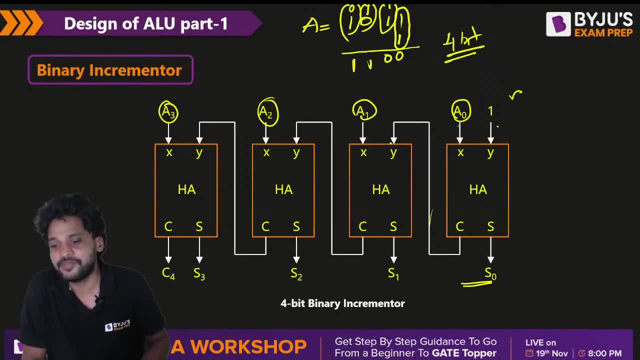 inputs. one is from a, one more is from the carry of the previous bit addition. so carry will be connected here and a1 is the next digit. a1 plus this, uh, c0. i would say a1 plus c0 will get connected, will be added sum will be produced here. carry will be produced here. so this is c1. 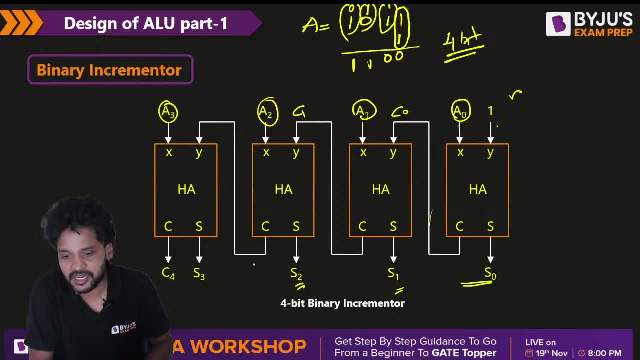 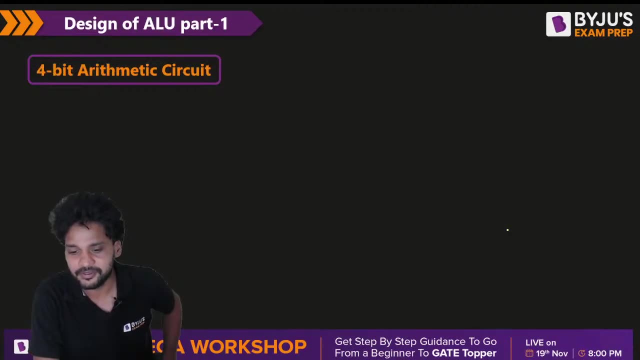 a2 plus c1 will get added. sum 2 will get produced here. carry will be added. a3 plus carry will be. the s3 will be here. c4 will be here. this circuit will simply be able to perform what incrementing operation. finally, what we going to do is: 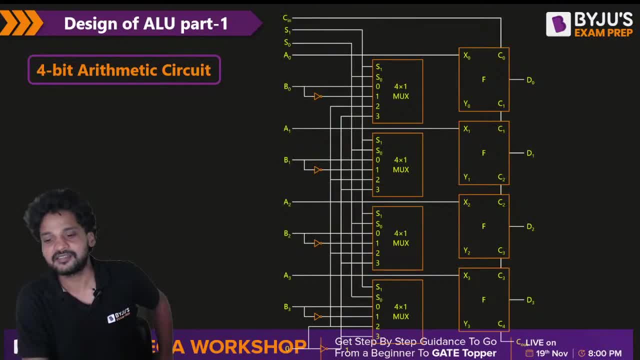 we are going to design a circuit which is going to perform, which is going to perform. am i here? are you here? yeah, in this circuit we are going to see. this is a circuit. what you are witnessing on the screen is a circuit which is going to perform addition. 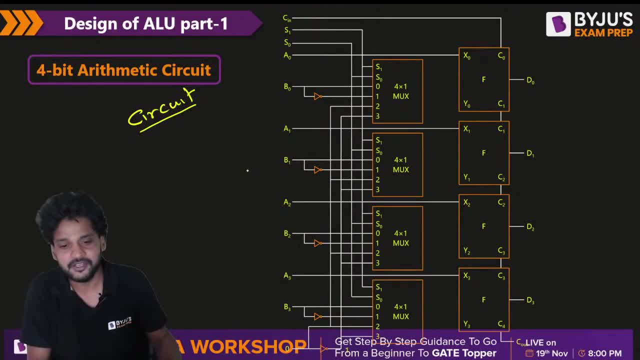 subtraction, incrementing and decrementing. so alu main part is arithmetic unit. right, this circuit will totally perform all the operations. so for what we have done: initially we perform addition operation. next, we designed a circuit to perform addition plus subtraction. then we, you know, design one incremental unit. finally, we need to design a unit which can perform addition, subtraction. 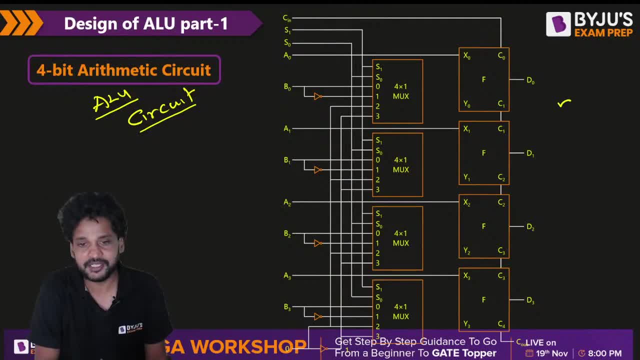 incrementing and decrementing- how? let us completely have a look at this circuit in order to demonstrate this circuit. stay focused carefully. in order to demonstrate this circuit, first of all understand it is the 4 bit alu. a 4 bit alu arithmetic units will have four full adders: full adder 1, full adder 2, full adder 3 and full adder. 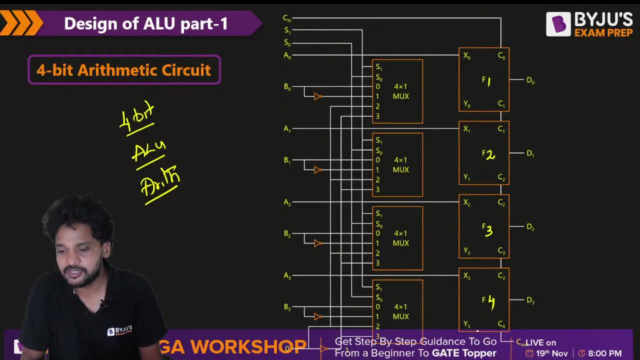 4. all these full adders will require a circuit which is going to perform addition incrementing three inputs. stay focused. full adder's first input is from a. have a look at this. there are three inputs. this is the first input. there will be a second input. second input: i did not show it. 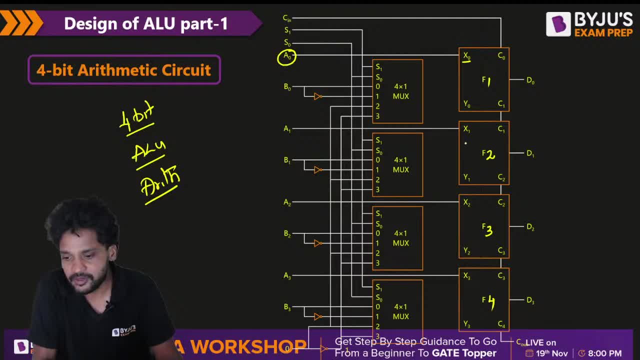 first input is from a. okay, look at this. there are four digits of a. i would say a is equal to 1, 0, 1, 1- least significant digit- a 0, next a 1. this is a. 2, this is a. 3, a0, a1, a2, a3 are connected to first full adder, 2nd. 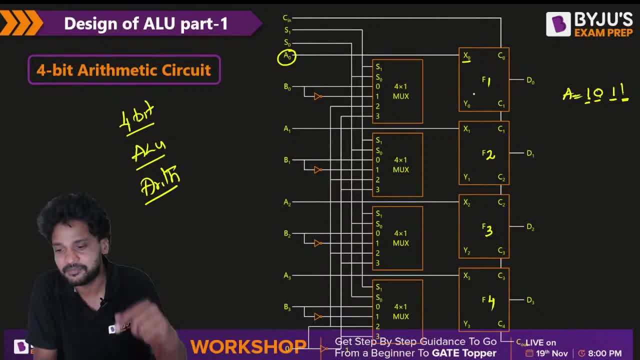 pull adder. third pull adder. 4th pull adder as the first input. you can see a0 is connected here, a1 is connected to. a2 is connected here. a3 is connected here. that means that every pull out of first input is taken from the digits of a. okay, now. 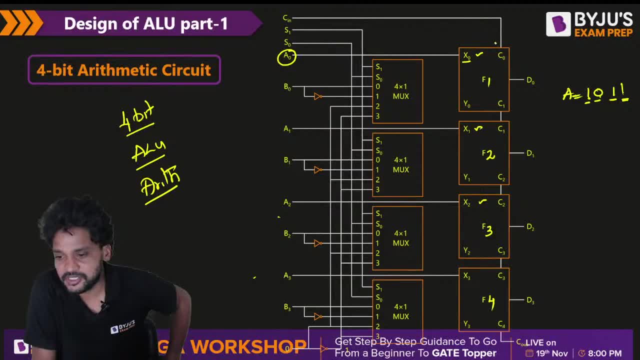 second input is not shown. third input is shown here. third input is from the external carry digit, this external carry digit exactly producing the third input. okay, now, what is the second input? second input is not. the second input has to be from b right, but b is not directly. 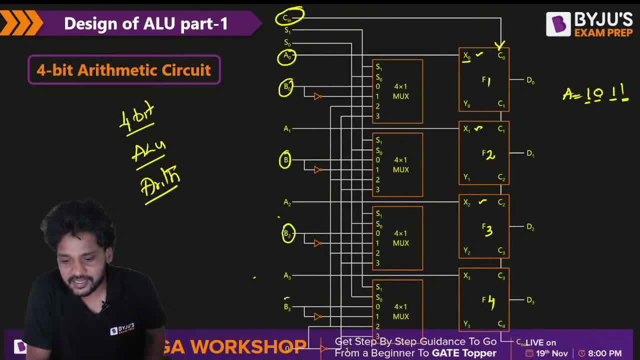 connected b actually is connected to the full add-on via a multiplexer. the second input of the full add-on gate: CLC car. yes sir, batch come start. which batch you're talking about Sunday? which batch you're talking about? if you can precisely ask me, I will. I will excuse the app. 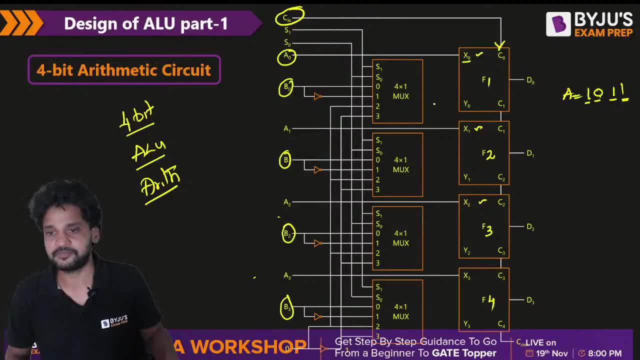 bash, or you know, the YouTube bash Sunday. ask me precisely, so that I will be able to answer now. second, input of the full add-on is the output of the multiplexer. it is already started. we are in the middle of that. we are in the middle of it. now the thing. 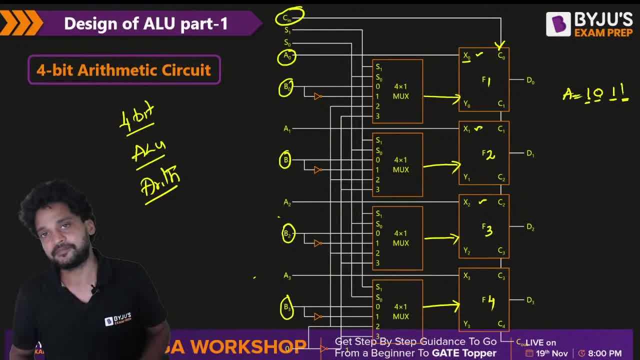 what's happening is the computer architecture and organization. okay, so, anyhow, not only this, we are coming up with the multiple sessions. this is one quick revision session. complete revision session. okay, the crash course. right, then we come up with what you call. there are some other plans. we we're going to tell you so. from this month to the next month, we are planning. 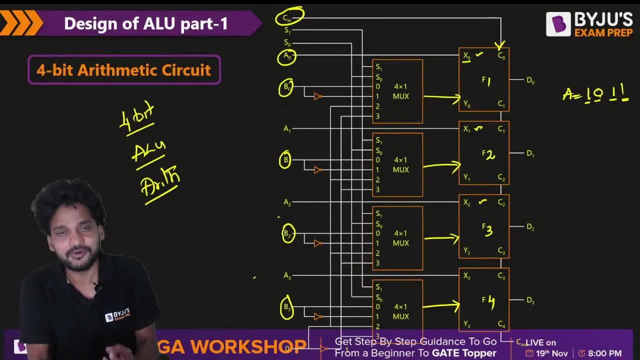 we already planned the crash course which is being executed right now. then we will come up with the marathon sessions. so do follow the YouTube channel regularly and carefully, so that you will be able to crack. anyhow, we are in the middle of the COE and the next session. I guess it is like. 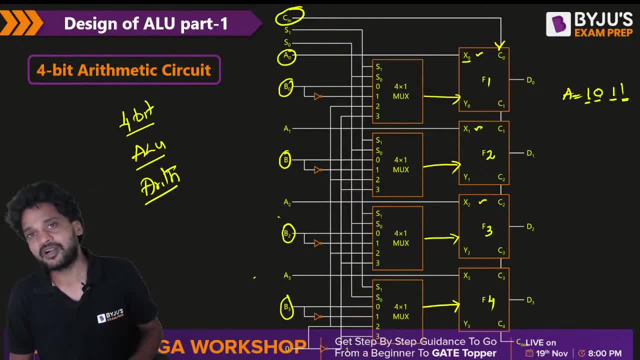 complete computer networks. I don't exactly know. I will let you know what is the next subject. okay, yeah now. anyhow, see, one input of the full add-on is from a. one more input from multiplexer. one more input from is the same. now, when you look at the multiplexer, the multiplexer is a four into one. 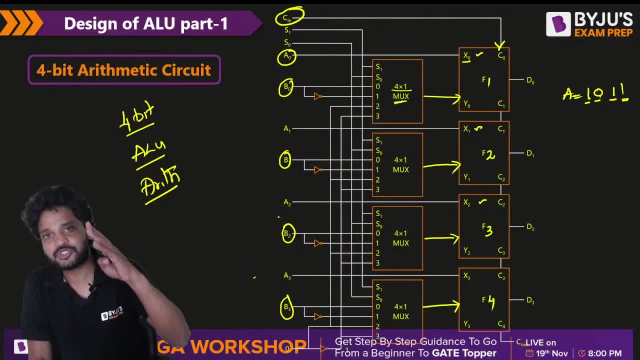 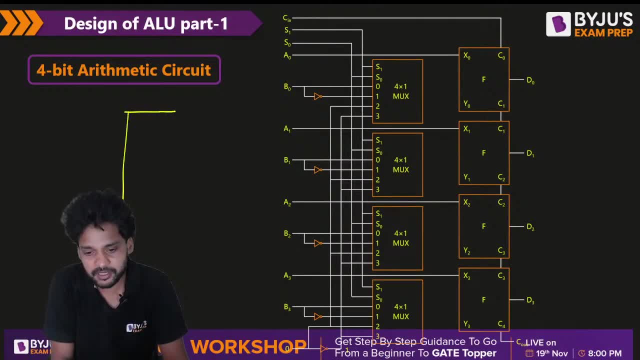 multiplexer. this four into one multiplexer requires four inputs. what are those four inputs? when you look at the multiplexer, I am drawing a blueprint of one multiplexer. okay, a four into one multiplexer. see, any multiplexer of this will have four inputs: one, two, three, four. 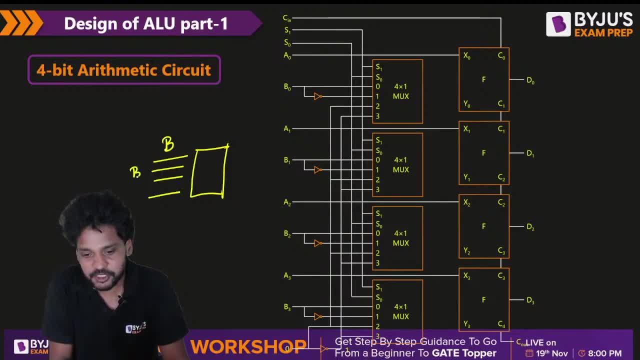 the first input is B. second input is B's complement. third input is zero. fourth input is one. look at this. first input is from B. second input is B's complement. third one is a zero, whether you are able to see this or not. the third input is zero. fourth input is one. similarly, go to the. 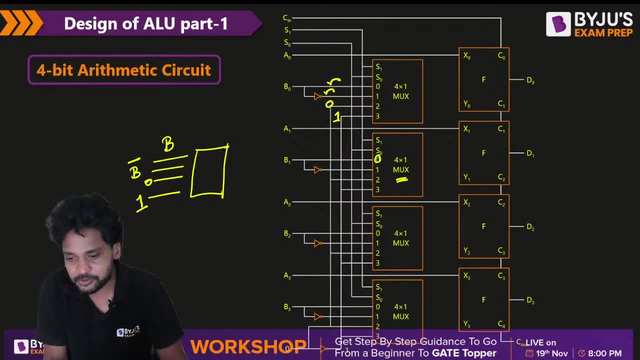 second multiplexer. the first input of the second multiplexer is B. the second input of the second multiplexer is B, complement. yes, the third input of the multiplexer is zero. fourth input of the multiplexer is one similarly B, B complement zero. one similarly B, B complement, and it is a zero. and 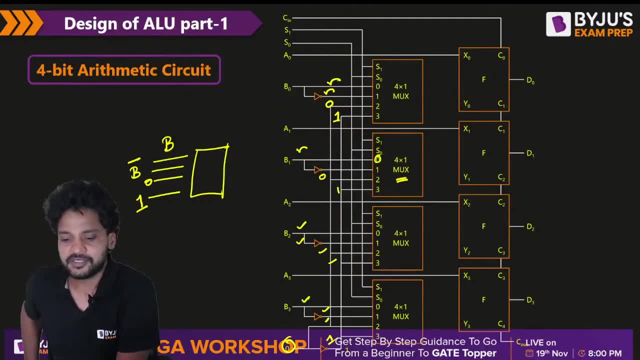 it is one. clear. okay, stay focused and understand. simple, understood so far. next, in order to understand operation, it is even more simple. there are common selection inputs to the multiplexer. which input is going to be enabled from the multiplexer side will be defined by the common selection inputs. you can see the selection. 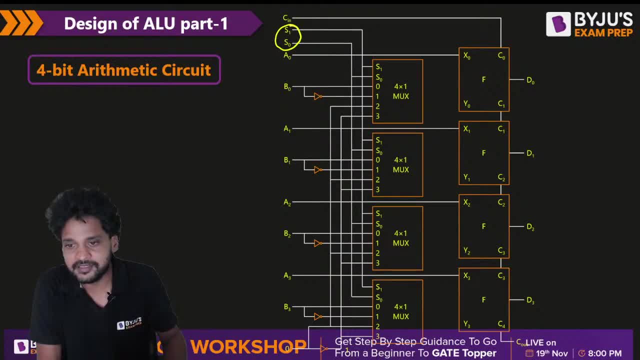 inputs: S0- S1. okay, S0 S1. no, no, it is not. AB01, Anuvaij. I understand. multiplexer is not connected from A input, XR is only connected. sorry, the full adder is only connected from the A input. you can see, A input is neither directly connected to anything, rather A input. 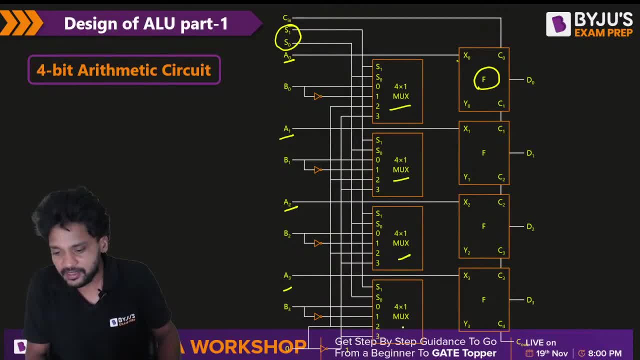 is never connected to the multiplexer directly. the A input, when you look at it, is directly connected to the full add-on. A is not bypassed. A is not connected via any channel. A is directly connected to the full add-on. yes, sir, no agreed or not? 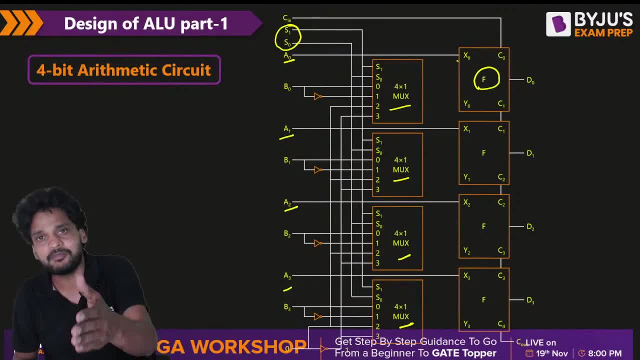 only B has been connected to the multiplexer. the output of the multiplexer is connected to the full add-on. this is precise to understand, okay. so now then let us understand. these are the selection inputs. these selection inputs are the common selection inputs to all the multiplexer. you can clearly see the selection inputs of the multiplexer are commonly taken. 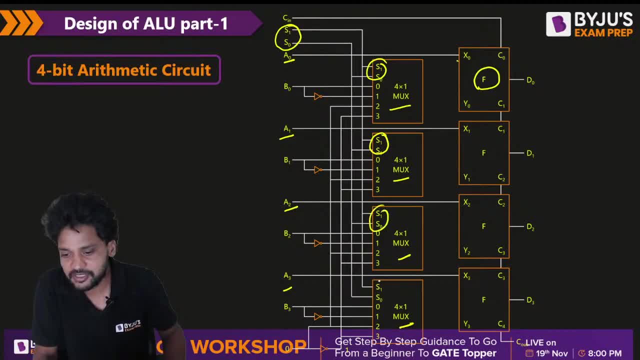 from these selection lines. these selection lines. okay, that means that the selection inputs are uniform to all the multiplexers. if the selection inputs are equal to zero- zero, then all the multiplexer selection inputs will be equal to zero- zero. now I will tell you how the circuit will be able to perform. 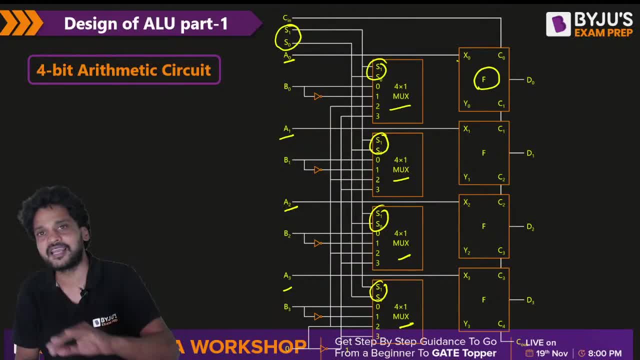 addition, subtraction, incrementing and decremented. so stay focused when the selection inputs are okay, fine. so if my selection inputs are zero, zero, what will happen? addition will get performed. why? because, see, multiplexer output is equal to B. multiplexer will enable the first input of it all. the first inputs of the multiplexer, needless to say, is B desert. 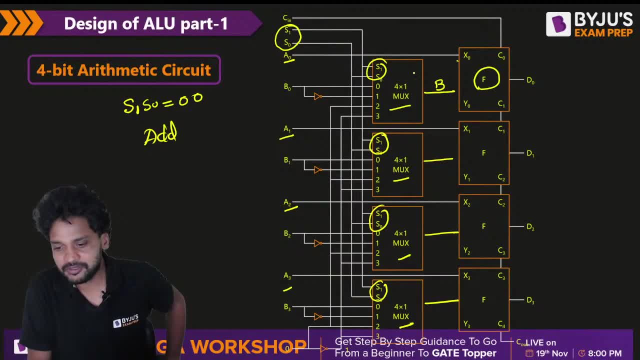 right, yes, sir, no multiplexer, whenever it receives the selection inputs, is equal to zero. zero. all the will enable their first input. The first input of the ALT multiplexer are the b digits only: b0, b1,, b2, b3.. Now what will happen? The full addo is going to perform the addition. 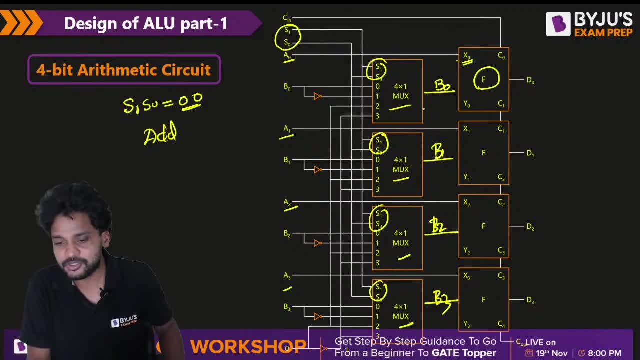 in between a, because a is already connected, and b. So during s1, s0, selection inputs are 0, 0, then the circuit is going to perform addition. And whenever s1 and s0 are equal to 0, 1, what is going to happen? Subtraction is going to happen. Why? Rule is, logic is: 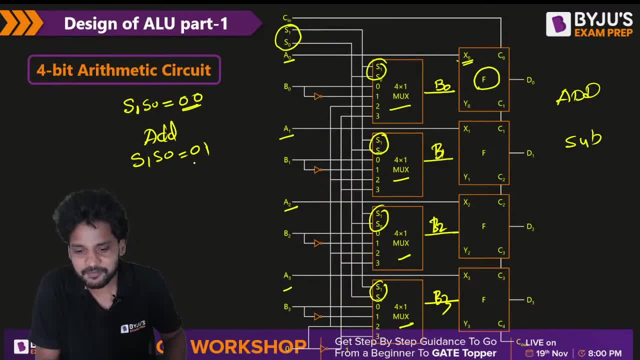 very simple, because whenever selection inputs are equal to 0, 1, what is going to happen? I will erase this. Multiplexer output is the second input. Selection inputs are 0, 1.. Second input will get enabled. What is the second input, Second input of the multiplexer is this complement Will crash. 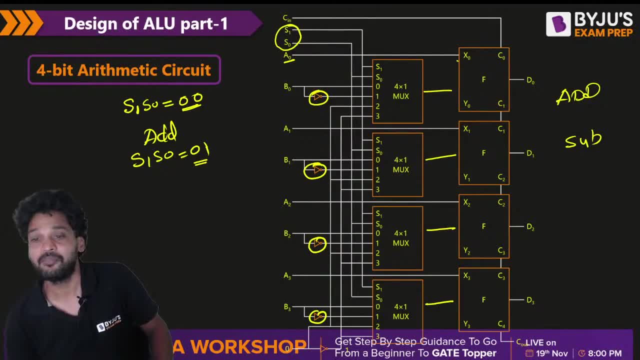 cores cover entire syllabus. Crash core covers important topics. Within 4 days or 5 days, entire syllabus coverage is a myth, but the important topics will be covered. But crash cores is supported by many courses that are coming up for you guys. You. 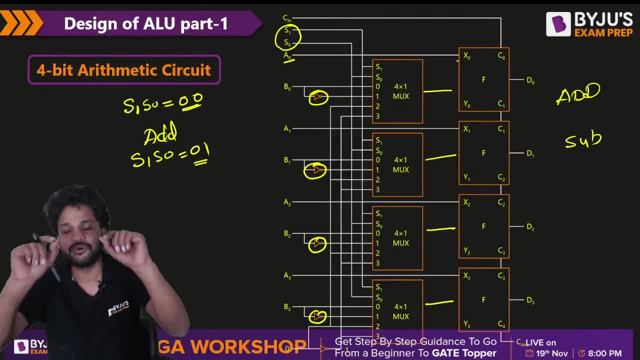 don't need to worry only about the crash cores. Crash cores is going to cover the important topics. Right, then we are going to come up with the marathon sessions. In the marathon sessions, we are going to make the total topic as comprehensive. Now, stay here. 0, 1 meaning. 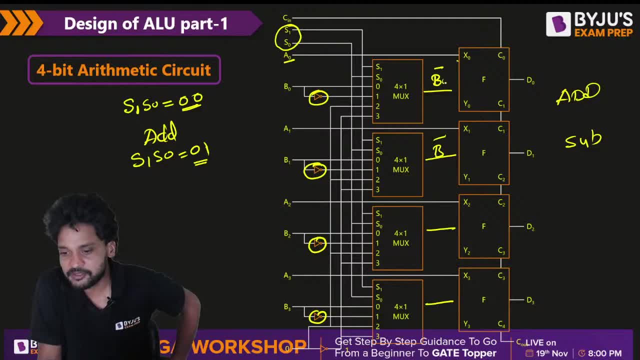 the second input of the multiplexer is 0, 1.. This is B complement. This is B0 complement, B1 complement, B2's complement and B3's complement. So all the B's complemented digits will be bypassed. So full adder is going to perform. 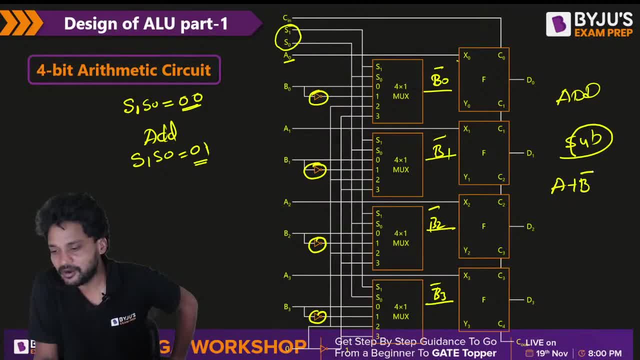 A plus B's complement. But in order to perform subtraction, I need to add, rather, I need to perform A plus B's complement plus 1.. A plus 2's complement of B is exactly equal to A minus B, Right? So in order to make it A plus B's complement plus 1, what I will do, 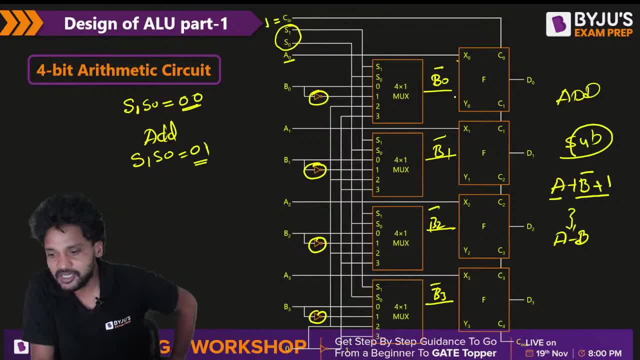 is. I will set the CN digit is equal to 1, because in the full adder A is 1, input B's complement is second input A plus B's complement is only half done. We need to perform one more addition of 1 digit. That 1 digit, that value 1, will be given from CN Whenever CN is equal. 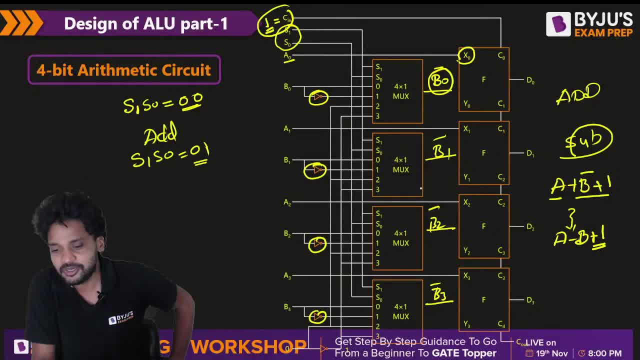 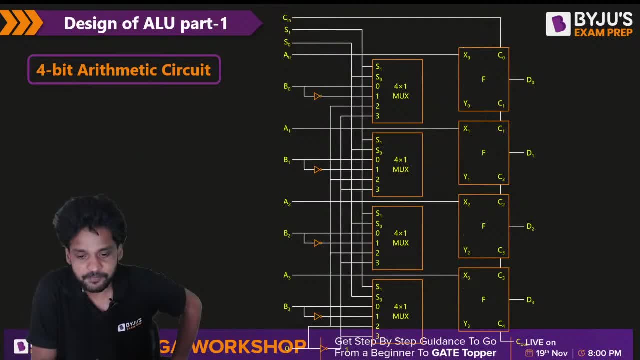 to 1 and S1, S0 is equal to 0, 1.. The circuit is going to perform subtraction. Okay, And the simple. needless to say, whenever S1 and S0 are equal to 1, 0, what will happen? The XR gate, third input, will get enabled. 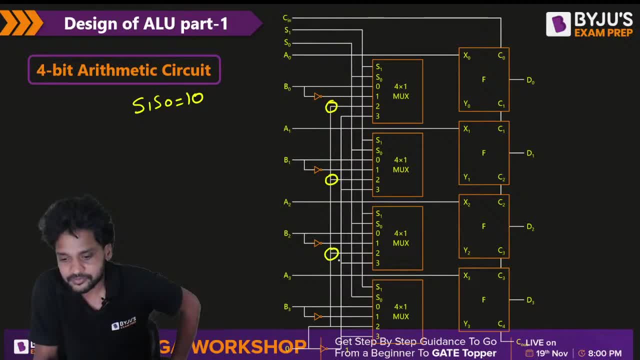 The third input of the XR gate is equal to 0.. The third input of the XR gate is equal to 0.. 0 will be enabled. Third input will be enabled and will be connected to the full adder. So full adder already got A and the second input is coming from the XR gate, The multiplexer. 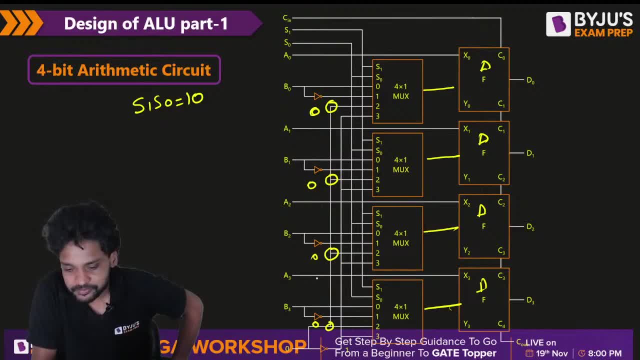 enabled the third input. The third input is 0.. Right, So the third input will be equal to 0.. The 0 is bypassed and connected to the full adder, So the full adder is going to perform A plus 0.. A plus 0 does not alter the value of A, So in order to make it A plus, 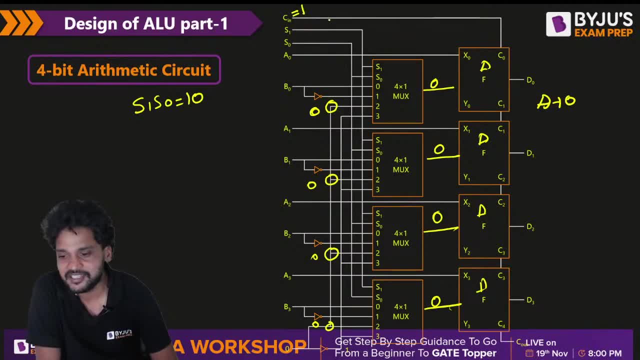 1, CN value, which is carrying digit, which is connected as the third input to the recall, full adder must be set to 1.. So at that time A plus 0 plus 1 will be performed. So here increment operation is getting performed. 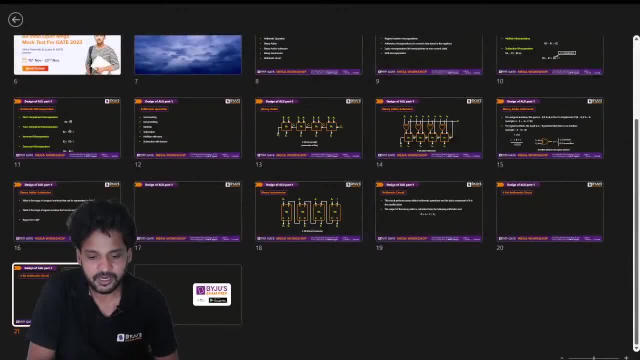 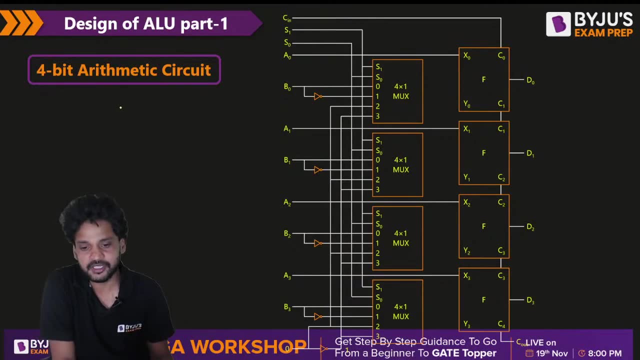 All right. Next thing, We have only one operation, that is, decrement operation. Now the thing is, Whenever S1 and S0 is equal to 1, 1, what will happen? The final input of the XR gate will get enabled. What is the final input? The final input of the XR gate is equal to 1.. So 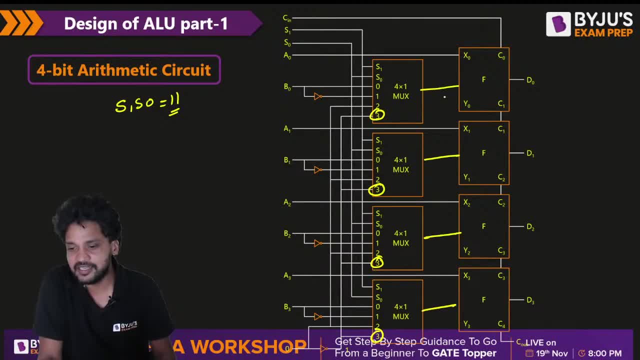 XR gate enable 1 and will send it to the full adder. Full adder is going to receive 1 from all the multiplexers. So here what is happening? A value- Let us say it is 1, 0, 1, 1 being added. 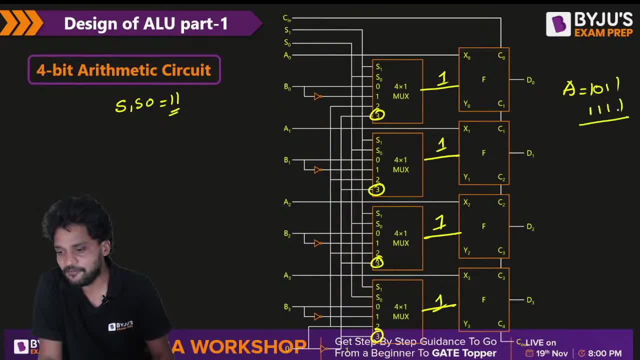 to 4 1's here. So how adding 4 1's to A is going to decrement the value of A. Understand carefully. This is the shortcut of decrementing. Stay focused and write it down somewhere When you want to decrement any register's contents. only the thing is you should be. 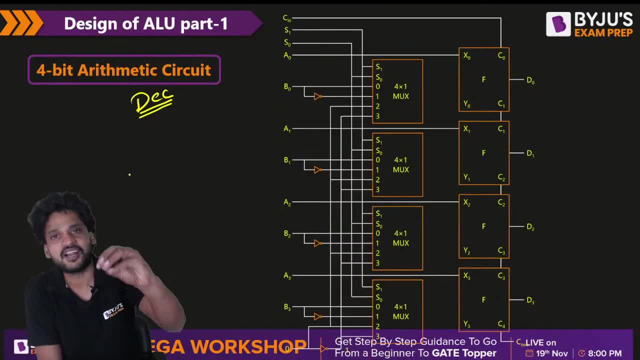 able to add those many 1's, which is equal to the number of digits of the register. For an example, I have a 4 bit register. If you want to decrement a 4 bit register value, you need to add 4 1's to the 4 bit register. There is a 6 bit register. You need to add 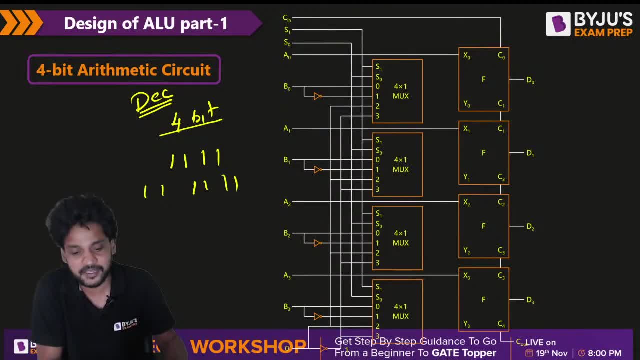 6 1's to the 6 digit register in order to perform decrementing. How it is going to happen? Understand There is a value: If there is a register, A register A is equal to 1 1 1 1.. When you decrement it, what will happen? 1 1 1 1 minus 1 is equal to 1 1 1 0. This. 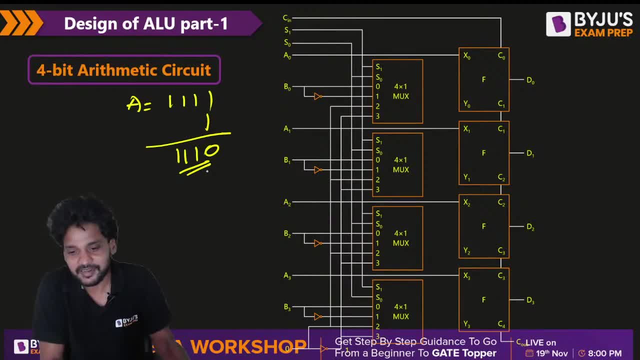 is how decrement is going to get performed. Right, But this is a regular decrementing. But in the computer you can't do it, You can't do it, You cannot do it, You cannot. When you want to decrement, what will happen is to the 4 bit value, 4 1s will be added. 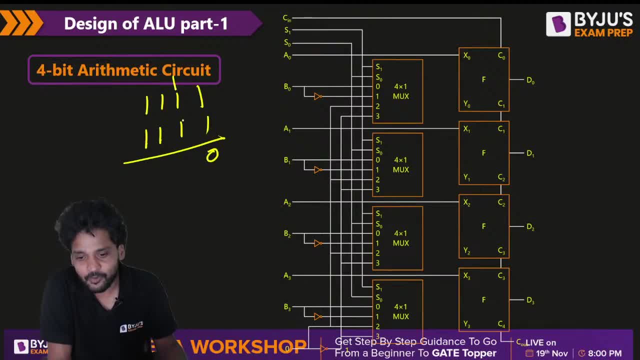 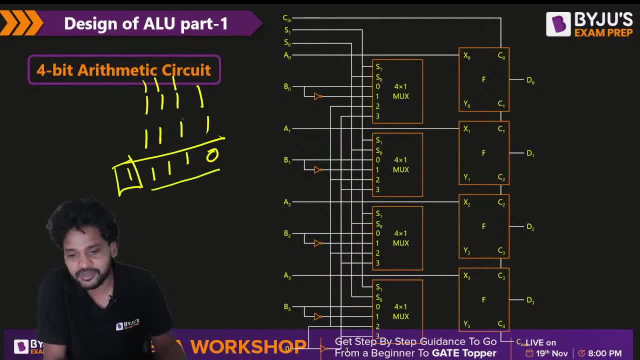 If you discard and carry triple 1, 0 is the exact value when you subtract a 1 from double 1, double 1.. Now I am going to take one more example. Let us think I want to subtract 1, 0, 1, 1.. 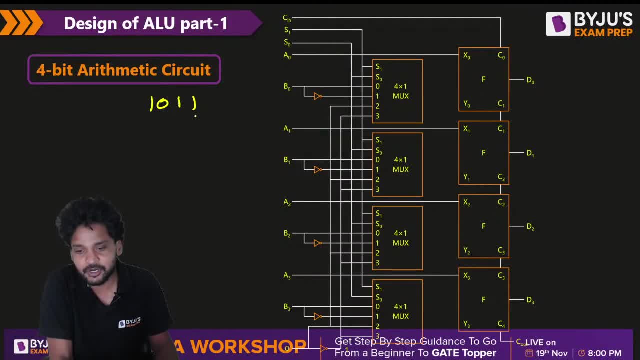 1 0, 1 1 must be subtracted: 1: 0, 1, 1 minus 1 is equal to 1 0, 1 0.. Right, We will see if this is going to work or not. So 1 0, 1 0 must be added with 1 1, 1, 1.. Clear. 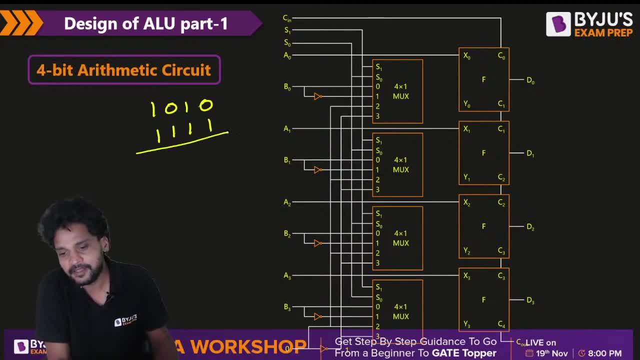 So what exactly is going to happen at that time? See, 0 minus 1 is not possible. 1, 0 minus 1 is equal to 1.. And I said: no, 1, 0 minus 1 is equal to. sorry, we are not performing, excuse me, got it. 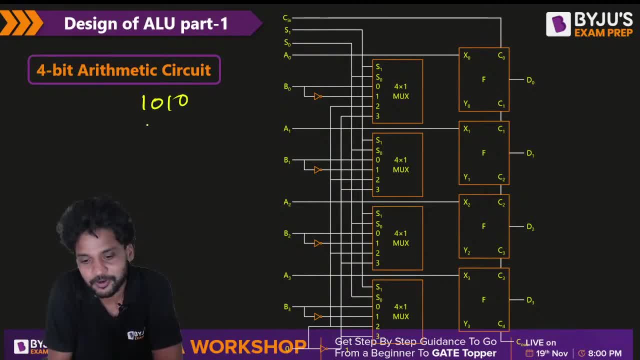 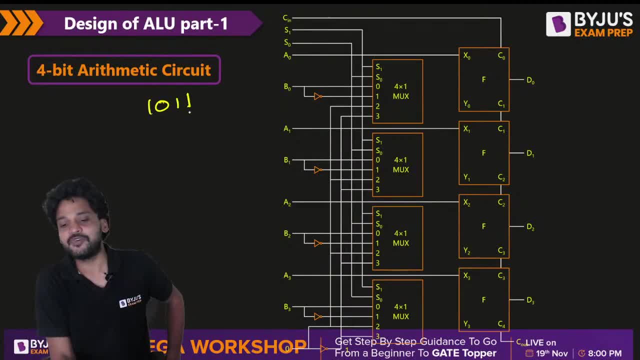 I guess it is 1: 0, 1, 1, right, Yeah, 1: 0, 1, 1 minus 1, bigger. pardon, I lost the track. 1: 0, 1, 1 minus 1 is equal to 1 minus 1: 0, it is 1,, it is 0,, it is 1.. 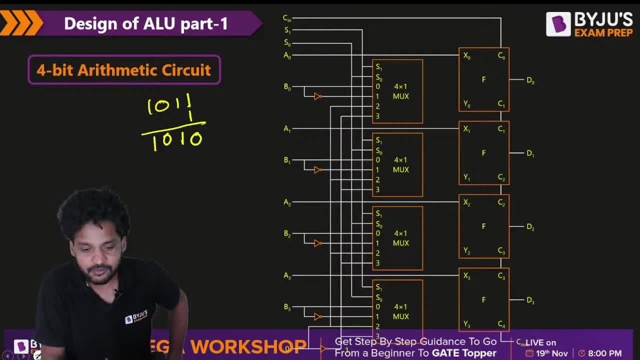 So it must be the value. So what we need to do is: what we need to do is to 1- 0,. 1, 1,. we should add 1- 1,, 1 1,, 4 1s. 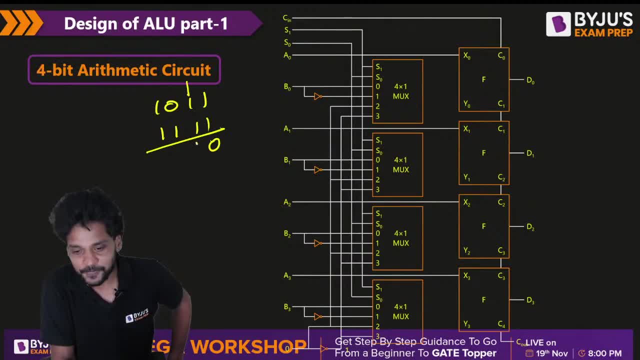 So 1, 1, 0,, yes, 1, 1, 1, 1, 1, 1, 1, 0. 1, 1, 1, 1, 1, 1.. So either you add 4 1s or you decrement, or you subtract, a 1.. 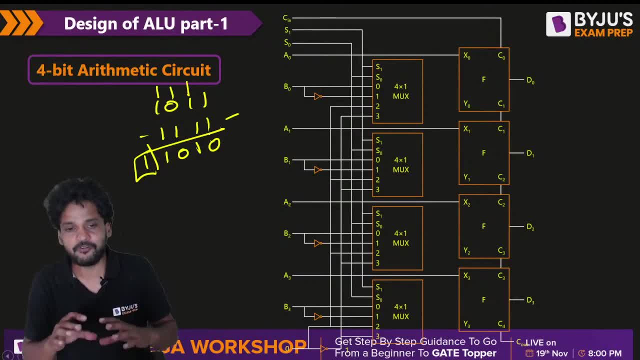 The things will be pretty same. So, in order to perform the decrementing operation, we should be able to add 4 1s to a 4-digit value. If it is a 6-digit value, you should be able to add 6 digits. 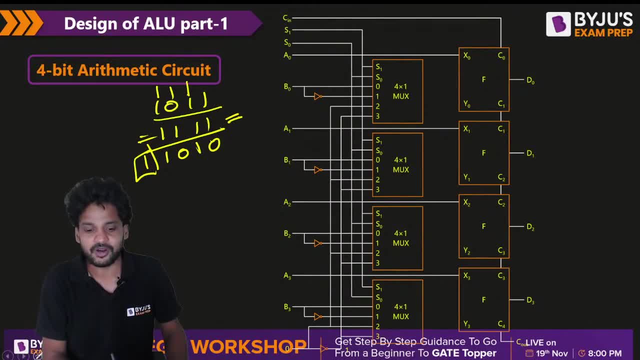 So here, So here, by the same rule, what we are doing is. what we are doing is, whenever selection inputs are selection input, where is selection? excuse me? yeah, s1 and s0 is equal to s1 and s0 is equal to 1: 1,. 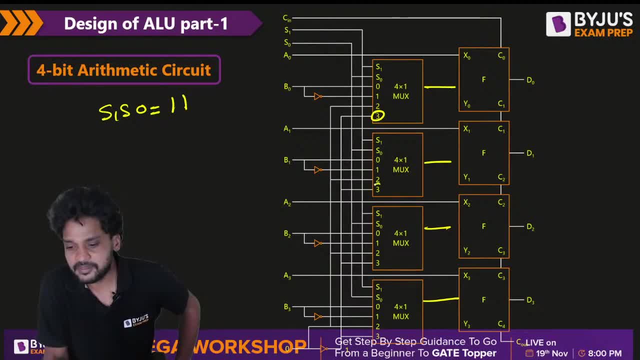 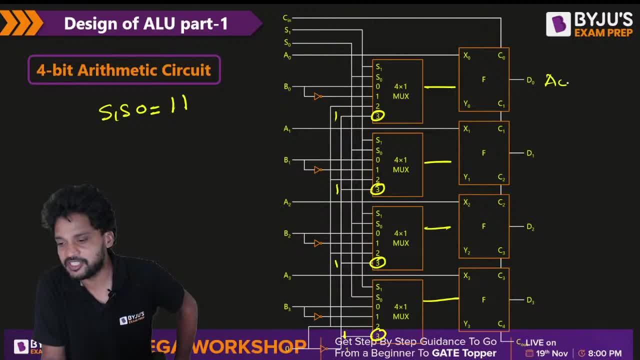 Already in the full add-on a value is available. This is a 0,, a 1,, a 2, and a 3.. Now all will get added with 4 1s, So that decrement operation will get performed. 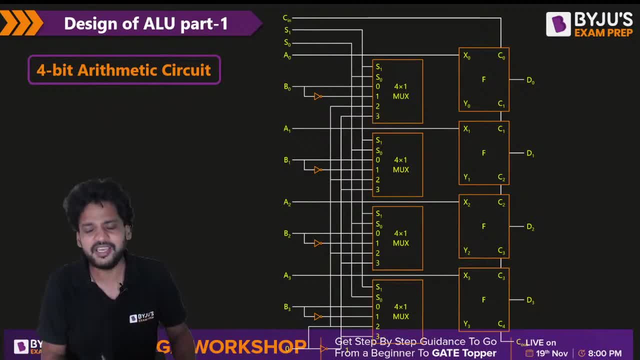 But here we need to understand why exactly decrement operation is being performed when we add those 1s. Reason is very simple: Because in the computer system when you want to perform a minus b, a minus b will be performed as a plus 2s complement of b. 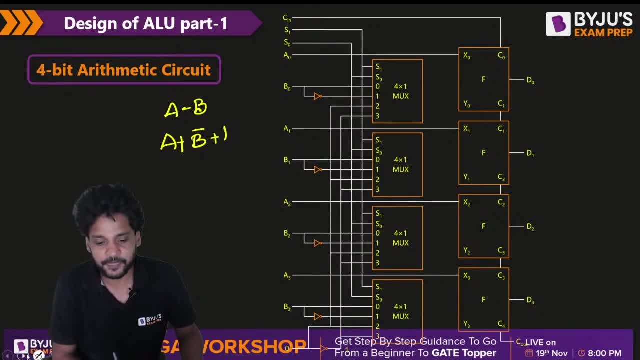 Right, a plus bs, complement plus 1 with this operation. So now thing is: let us say I want to perform a decrement operation: 1, 0, 1, 1 minus 1.. Did you get it Now? here, this 1 will be considered as b. 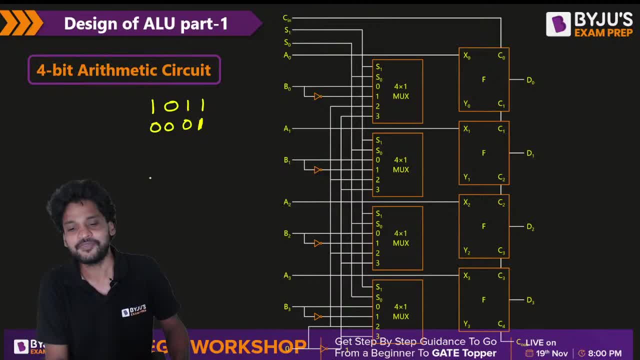 b will be equal to triple 0, 1.. Yes or no, a is equal to 1 0, 1. 1 should be subtracted Rather. a 1 must be subtracted from 1 0, 1, 1.. 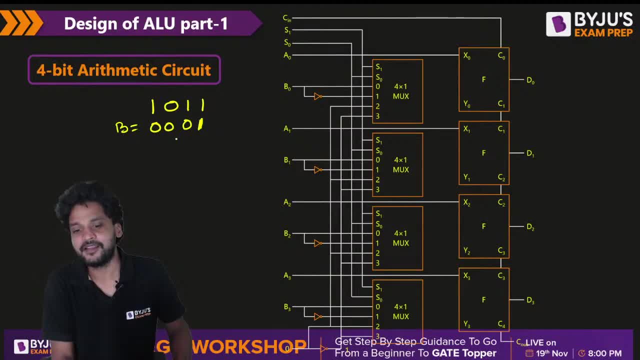 So b becomes triple 0: 1.. Now we need to convert this into its 2s complement Initially. please convert into the 1s complement. 1s complement of triple 0: 1 is equal to triple 1: 0.. 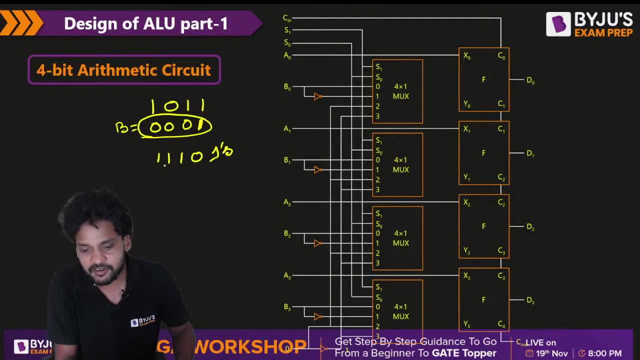 This is 1s complement 2s complement of triple 1: 0 is equal to 1s complement plus 1.. That is equal to 1 1, 1, 1.. This is the reason why, whenever you want to subtract a 1,. 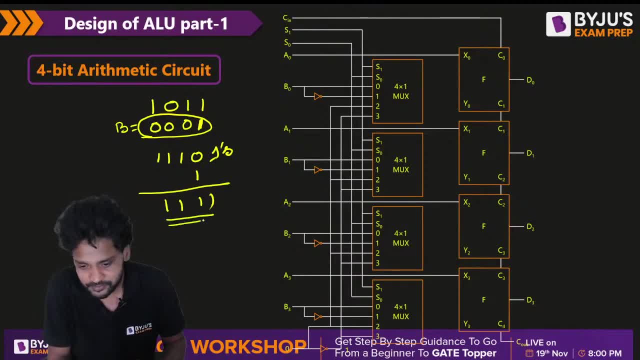 finally, we will get 1 1 1, 1.. Okay, So this is the 2s complement of b, which is equal to triple 0, 1.. So when 1 1 1 1 gets added, actually we are performing a plus bs complement plus 1.. 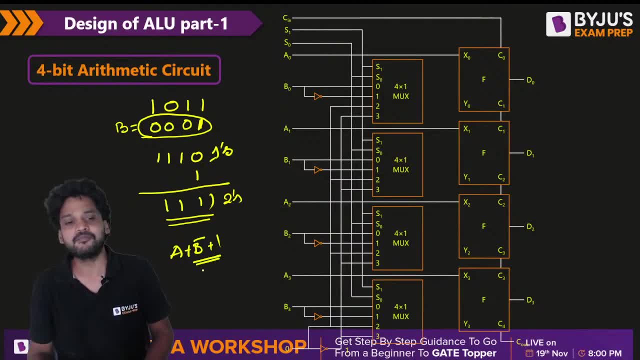 2s complement of b. only Right. We are not moving anywhere outside. We are exactly confined to the semantics of the processor. I hope I made my point very clear here. Even decrementing also is equal to subtraction. Subtraction, there is only way possible. 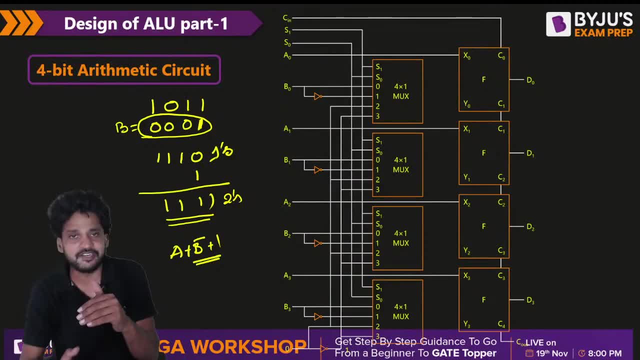 First of all, we need to take the subtrahend, We need to convert it into 2s complement, Then add it to the minion, So minion plus subtrahend's 2s complement plus 1. Sorry, subtrahend's 2s complement. 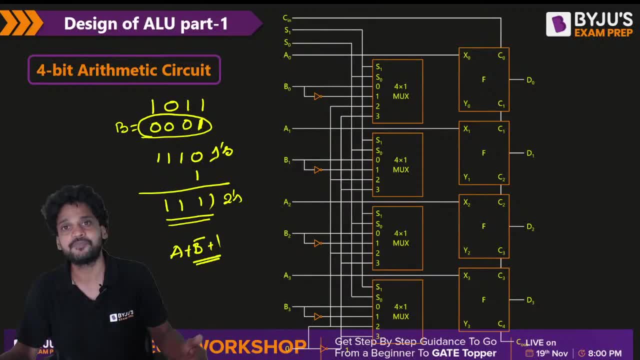 We will be giving you a minus b. As simple as this. Okay, With this, we have designed an arithmetic unit of the system. Understand carefully, Understand carefully. This arithmetic unit is capable of performing addition, subtraction, incrementing, decrementing. 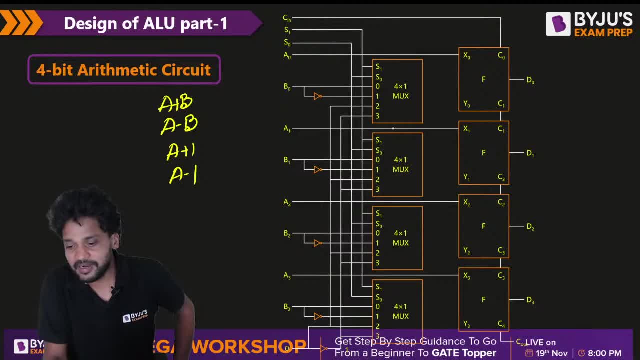 But for this the multiplexer inputs must be equal to. for the addition, it must be 0, 0.. Selection inputs- I am talking about S1, S0- must be equal to 0, 0. And S1, S0 must be equal to 0, 1 for subtraction. 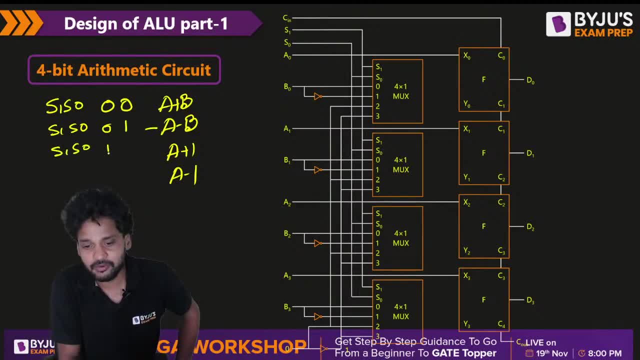 Okay, And S1, S0 must be equal to 1, 0. Whenever S1, S0 are equal to double 0, this circuit is going to perform addition. Whenever it is equal to 0, 1, subtraction is going to get performed. 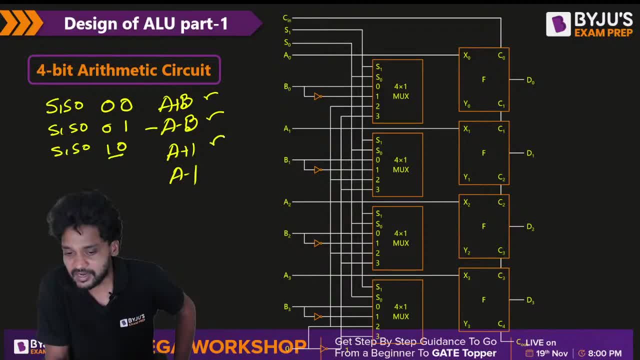 Whenever it is equal to 1, 0, incrementing will get performed. Whenever S1 and S0 are equal to 1, 1, decrement operation is going to get performed. Clear, Now hold on. We did not completely finish it. 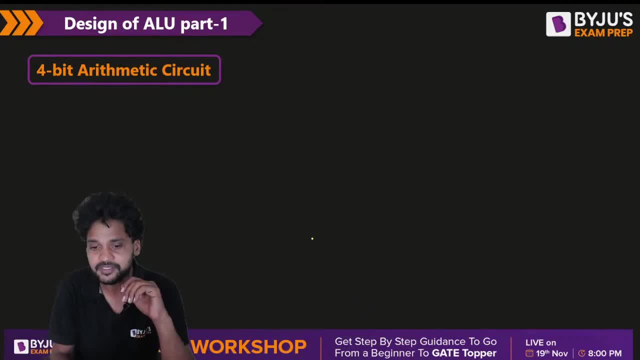 As I told you. let me go back See. The ALU is a multiplexer unit of Multiplexed unit, of arithmetic units, logic units and shift units. Okay, How to design logic unit and shift unit? We do not need to worry. 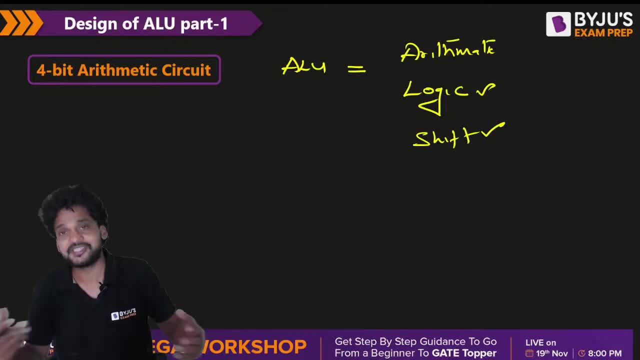 We do not need any different what you call. you know the design mechanism. The design mechanism can be very simple for logic unit and shift unit. For performing shift, it is even more simple: Use a shift register. Use a shift register. 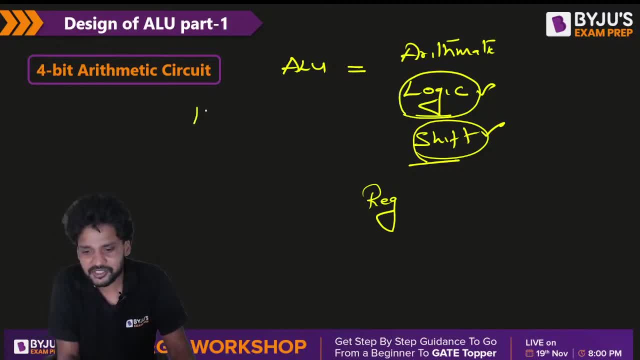 And for designing the logic unit, understand. there are 16 logic operations. Each and every logic operation is supported by a corresponding gate, Except a few logic operations. let us some. logic operations are clear and such. For this, like you know, we do not need any gates. 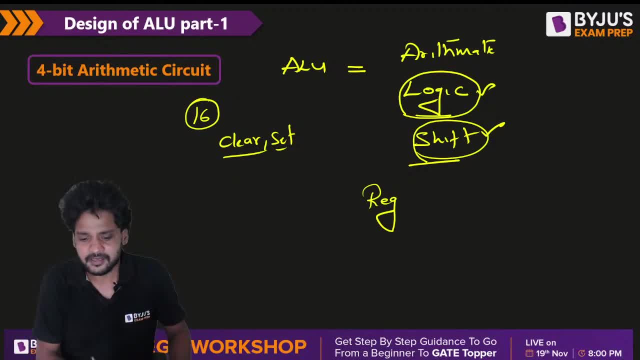 Rather, some other mechanism is actually required For that. understand carefully How to design the logic unit. All the 16 operations will be multiplexed. I will use a 16 into 1 multiplexer. All the corresponding gates will be connected as the inputs to this multiplexer. 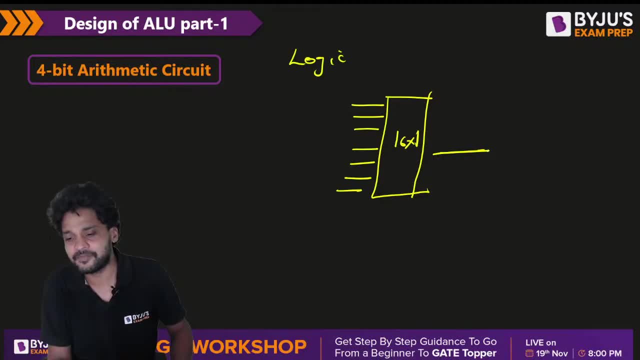 Then there will be output generated from one of the inputs. Let us say: this is AND this is, OR this is NOT. So a logic unit of an ALU is the multiplexer unit of all the logic operations. Now, what is the shift operation? 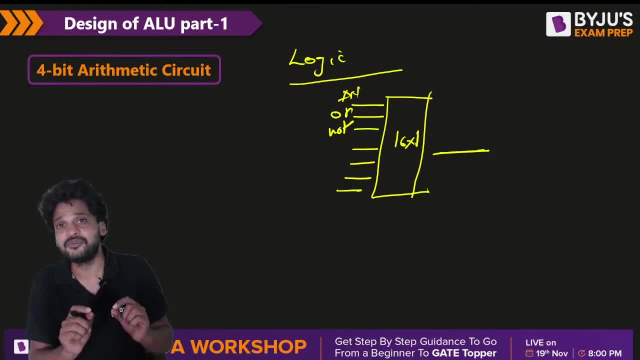 In order to perform the shift operation, I just require to use the shift register. Now let me show you the complete ALU. The complete ALU is the multiplexer unit. It is a 4 into 1 multiplexer unit. Okay, 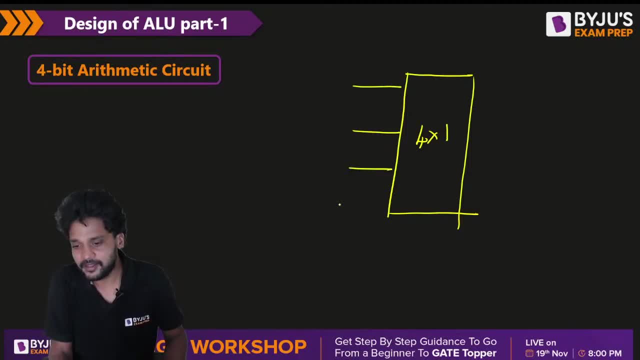 It requires 4 inputs. Okay, Now, if you remember, I have 3 units in the system. One is arithmetic unit. The arithmetic unit output is connected to the first input of the multiplexer. The logic unit output is connected to the second input of the multiplexer. 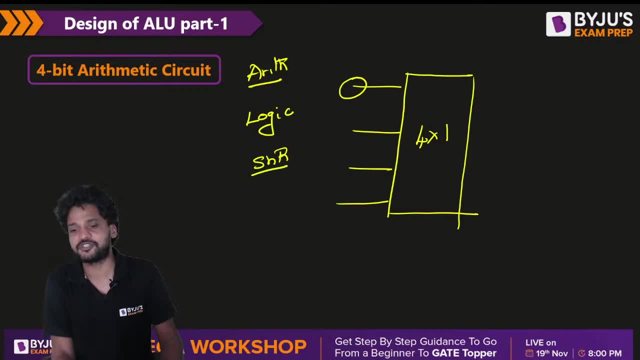 And shift right. I will use the shift right shift register. That will be connected to the third input of the multiplexer. Got me Shift left. that will be connected to the fourth input of the multiplexer. Now, this is my design of the ALU. 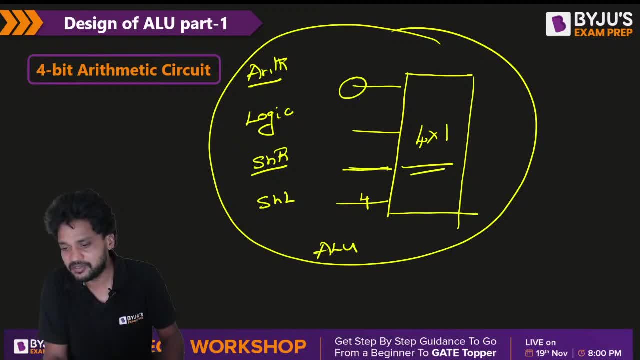 We will take 4 inputs. It is a multiplexer unit. 4 into 1. multiplexer Once again. first input is from the arithmetic unit. What is arithmetic unit? Just a short while ago we designed the total arithmetic unit. 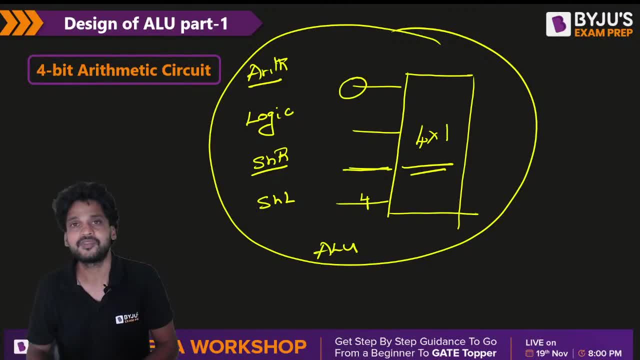 The output of the arithmetic unit is connected to a 4 into 1 multiplexer, which is the final multiplexer of the ALU. The output of the logic unit is connected to, again, the 4 into 1 multiplexer. Similarly, shift right and shift left. 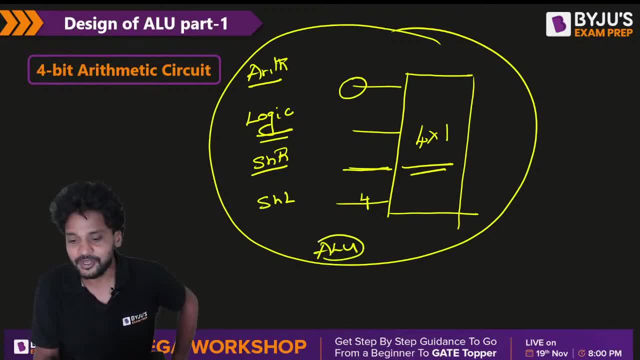 So this is my total ALU, which is going to perform all the operations. Any operation, one at a time, It can perform. if I am an ALU, I can perform a wide variety of operations. I can perform 6 arithmetic operations. 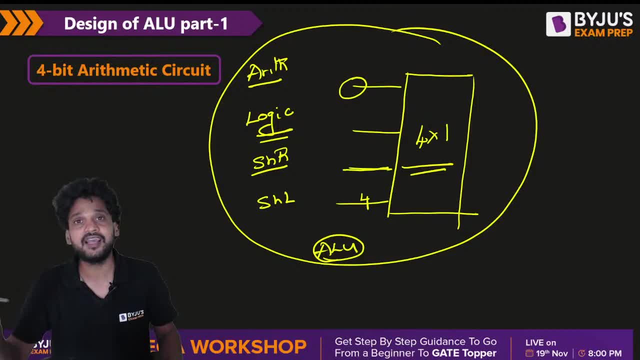 Addition, subtraction, incrementing and decrementing. Addition with carry. subtraction with borrow: 16 logic operations, 2 shift operations- Right shift and left shift- But only one at a time. I can't execute multiple operations. ALU can perform any operation from arithmetic logic- shift, right, shift, left- but only one at a time. 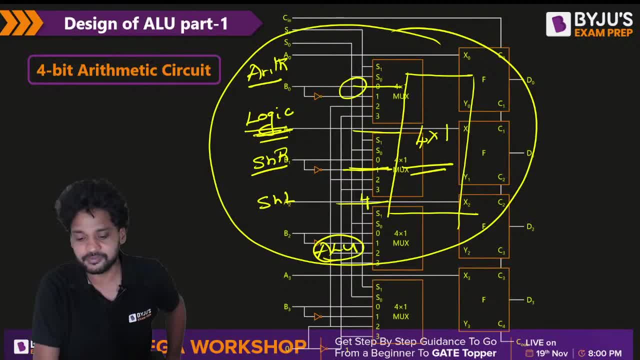 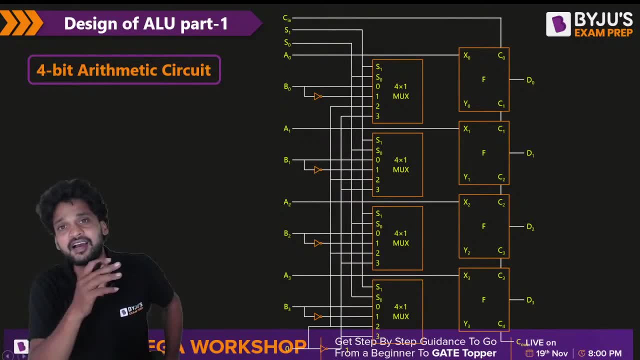 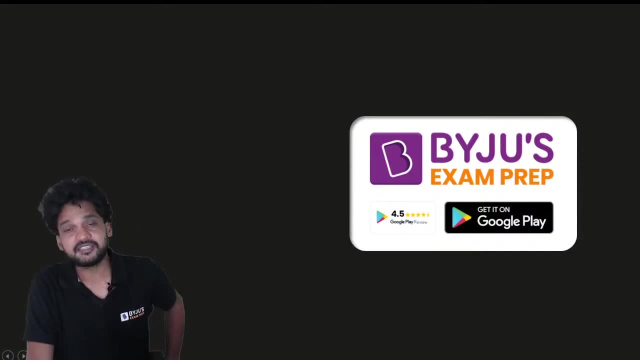 Okay, So with which we have come to an end of this session. I hope you got it comprehensively understood Till the way I intended you people to understand. Okay, I request you people to like and share the session And subscribe to this channel if you haven't already yet. 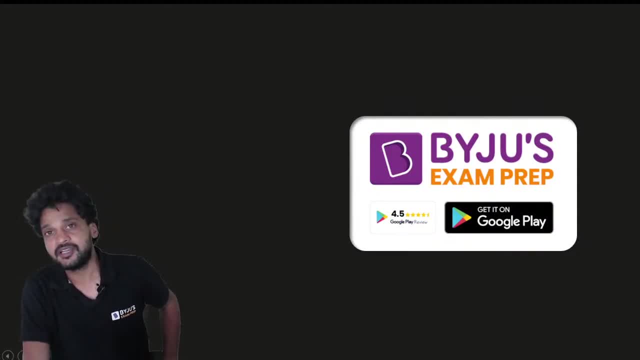 Unless you do have any follow up questions, Anil Prasad Swarampudi is going to sign off. Thank you so much, And that's it from this session. If you do have any doubts, ask me right now, in the next 2 minutes. 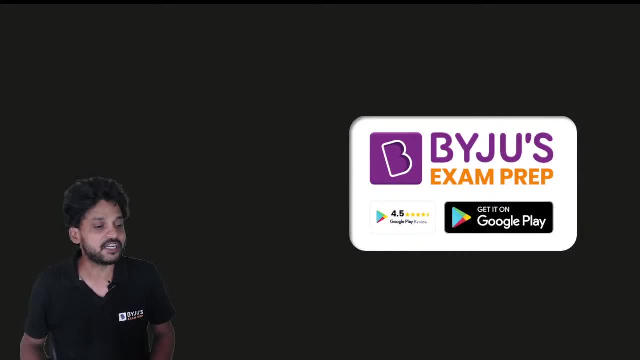 Otherwise we are going to, you know, finish this session straight away. But once again, let me admit firmly: it is the time for you people to get the mock test. Mock test is on your way, from 15th of this month to 22nd of this month. 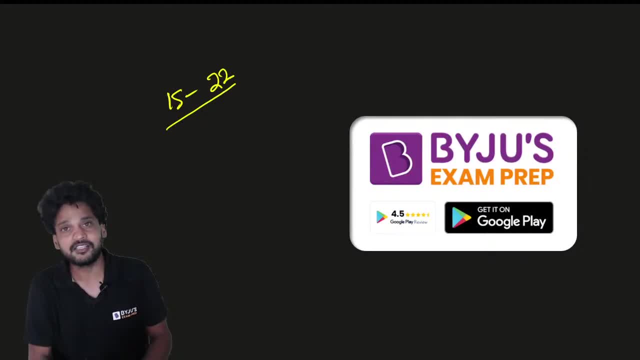 Please attempt this mock test without fail. This mock test is very important in deciding your GATE rank. When you give this mock test, you will be able to know where exactly you are standing in. You will be able to clear or cover all the loosens. 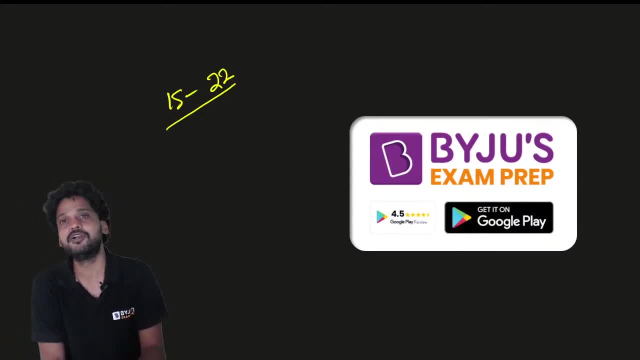 You will be able to prepare well And then you will be able to get a very good rank in the GATE. Okay So, and one more thing is there is one excellent session from Abhinav Nageshwar is coming on your way live from 24th of this month. 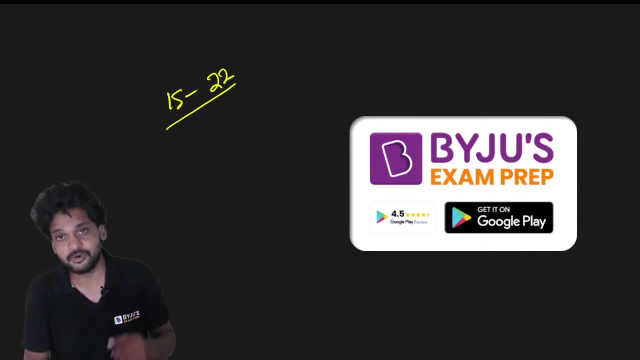 Okay, At 8 pm. So don't miss this opportunity because you are going to get every tip and trick in the world to crack the GATE exam. Okay, Keep in mind all the operations performed. Operations are not performed using multiplexers. 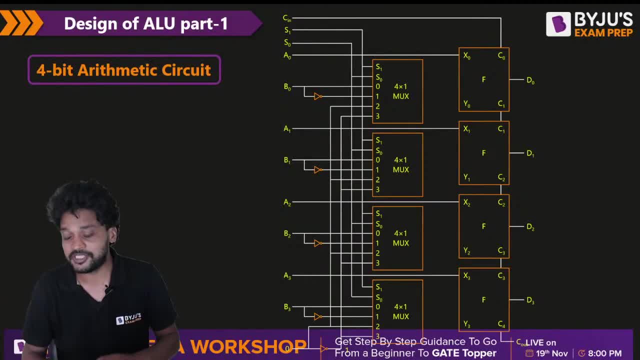 Do not get. Operations, sir understand, are performed in PULADAR. only Right Operations will be performed in the PULADAR. if it is the arithmetic unit, Operations will be performed in the GATE. The GATE is the logic unit. 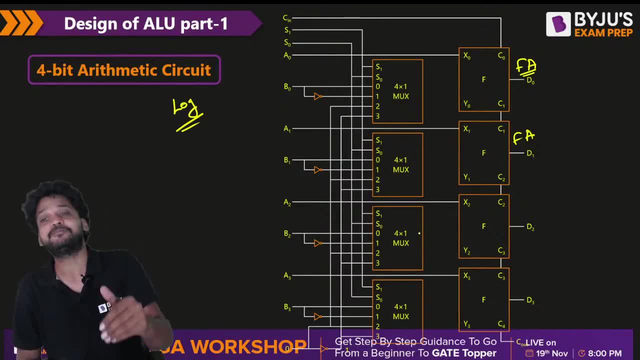 But multiplexer will select. Multiplexer will select only one operation. Understand, Did you get my point? Let us say: look at this unit, Stay focused. Look at this unit, See This. multiplexer can select one of the B inputs. 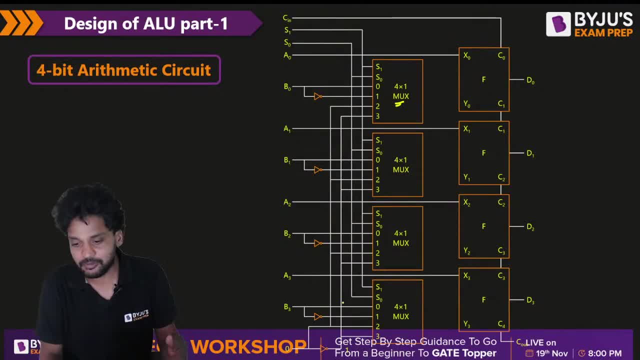 Got me. So according to the multiplexer's inputs, one operation will be performed. Got me The PULADAR. So if it receives B, A plus B will get performed. Okay, If it receives B's complement, A plus B's complement will get performed. 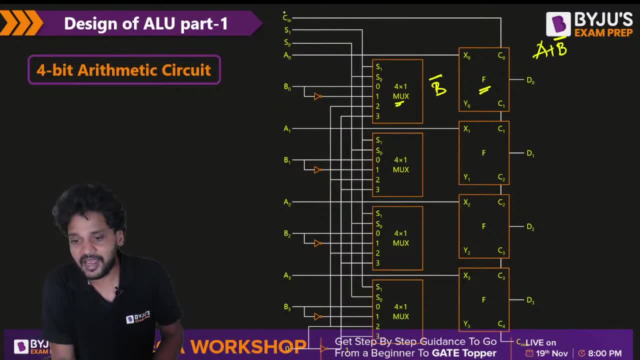 So, in order to make it A minus B, we will add a 1 from Cn, We will make Cn is equal to 1.. So A plus B's complement plus 1, needless to say, A minus B. 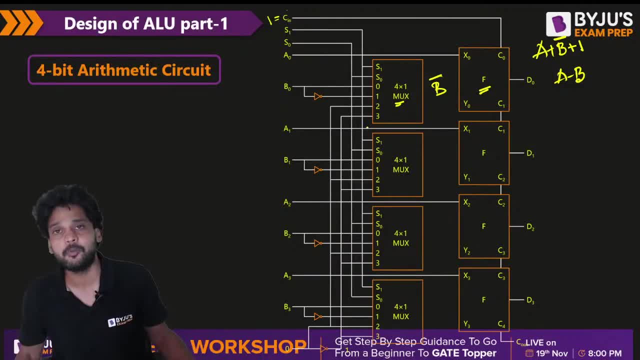 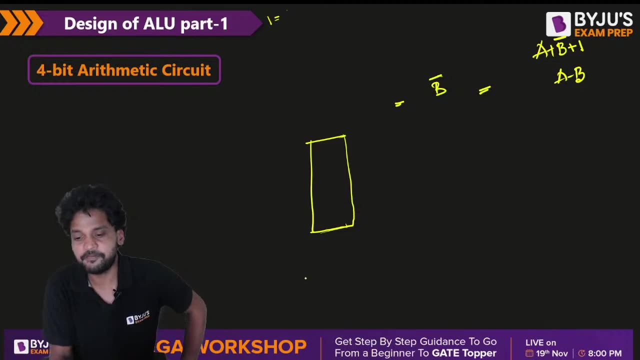 Did you get it? Multiplexer is not performing any operations, Rather even for logical. stay focused, Even for logical. even for logical. see, there is like an OR gate, There is an OR gate, There is an AND gate. 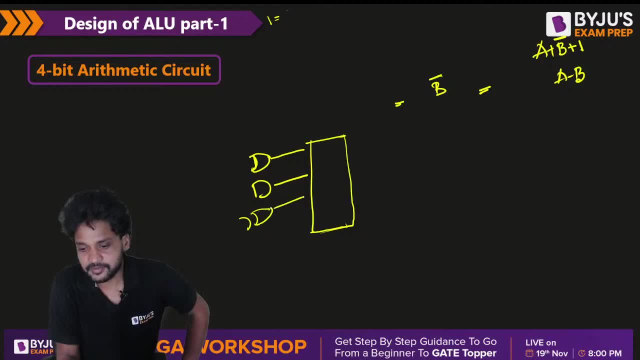 Okay, There is an XOR gate And there is a NOT gate. I hope you got my point. Okay, Now understand. I have two inputs. One is A, One more is B. A and B are applied to all the gates. 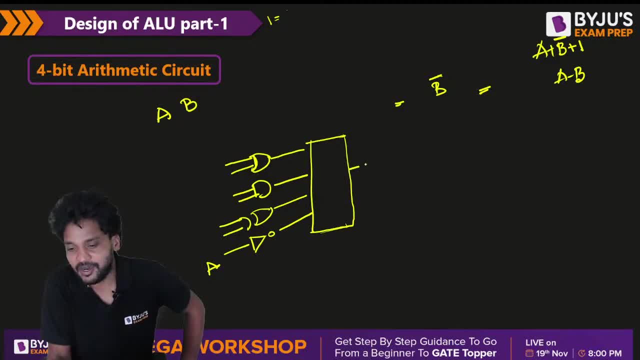 But for the NOT gate, only A will be connected. Now it is the selection inputs of this multiplexer. S1, S0 will define and decide which operation is to be performed. Did you get it Now? S1 and S0 are equal to 0, 0.. 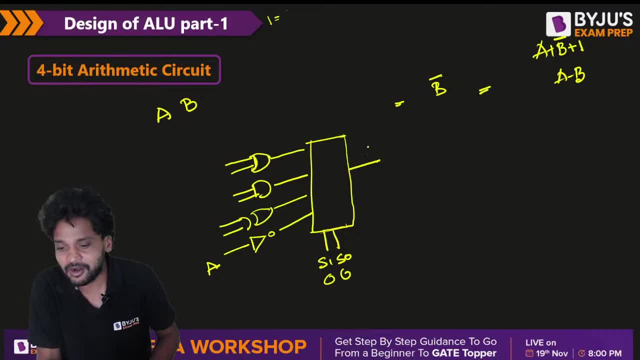 So the multiplexer is going to perform what you call OR operation. Multiplexer is going to enable OR operation because, understand, OR operation is being only performed in the OR gate, But the multiplexer is selecting the OR operation. It might make my point very clear. 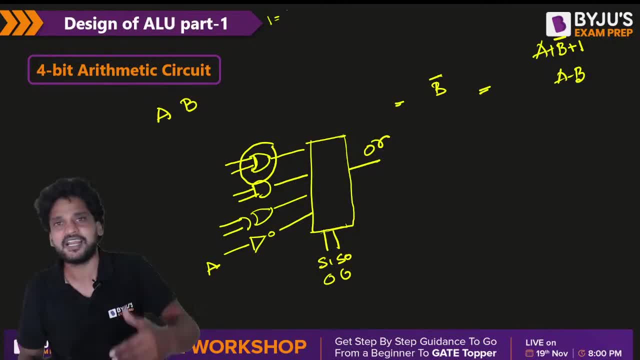 It might Multiplexer is not. It is only for selection. Already I am a multiplexer. I am receiving four inputs: One is from OR, One is from AND One is from what you call XOR, And one more is from NOT. 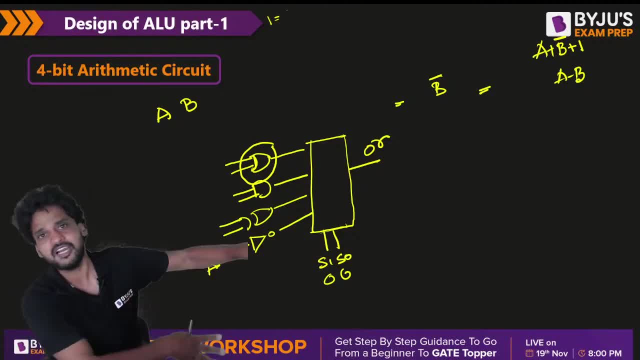 According to my selection inputs, the operations are already performed and the outputs are available at my inputs. I will select one input. I will send as an output. Got my point? I am not performing any operation, rather than selection. Did you get it? 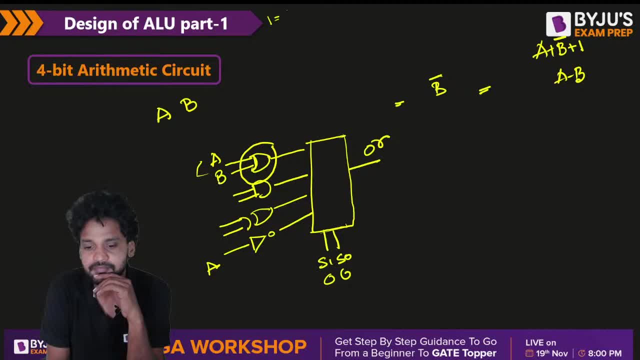 In my. Do I have you with me? Is your doubt clarified? Okay, So we need four into Four, sixteen into one, multiplexers for performing all logical operations on. Yes, Correct, What you told is correct Here. you spotted a very good point even before I tell you. 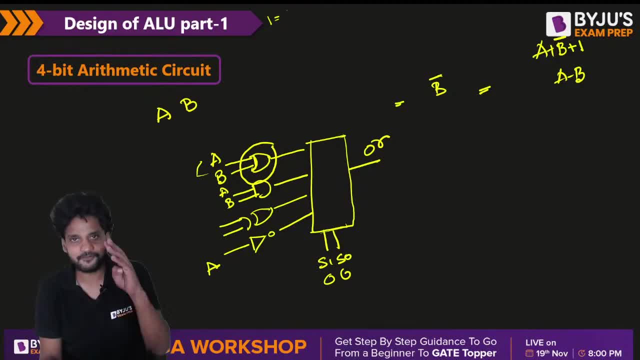 We need four stages. Right, We need four stages, But actually because of the limitation of the screen, we are just able to see only one stage Like that. we require three more stages. I hope you got that point already, Right? 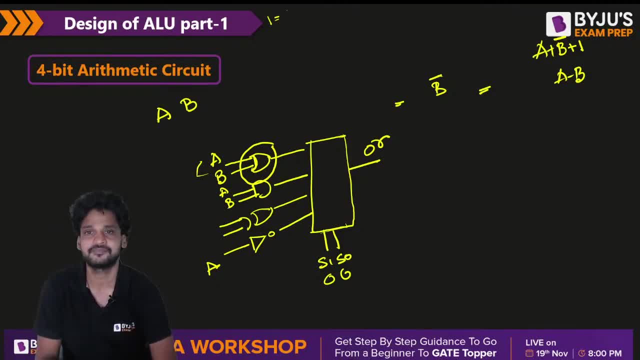 Absolutely, you are correct. Absolutely you are correct. You are perfectly spot on. Anu Ajay, did you get his point Here? yes, There are. Let us say: A is a four bit value, B is a four digit value. 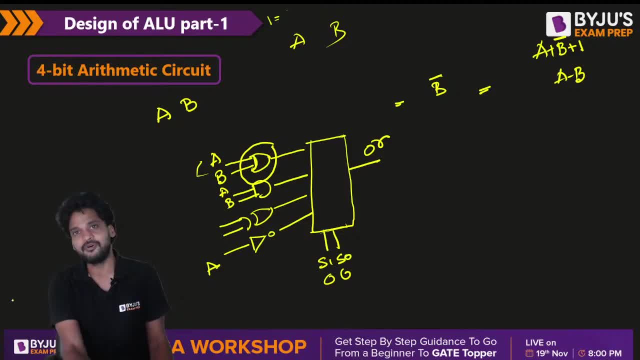 Now like this: I will require you know four more stages. Right Here, we will be able to show only one stage of the ALU. Okay, Like that, but there are different stages. This is only for the first digit, A0, B0.. 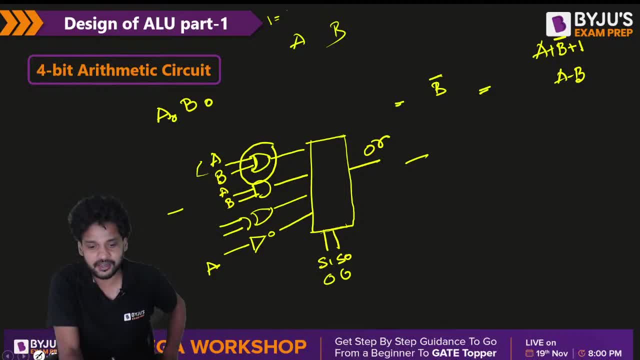 But there is A1 still. Let me erase this. Okay. A0, B0.. For A0, B0, this is the first multiplexer, But still there is A1, B1.. Still there is A2, B2.. 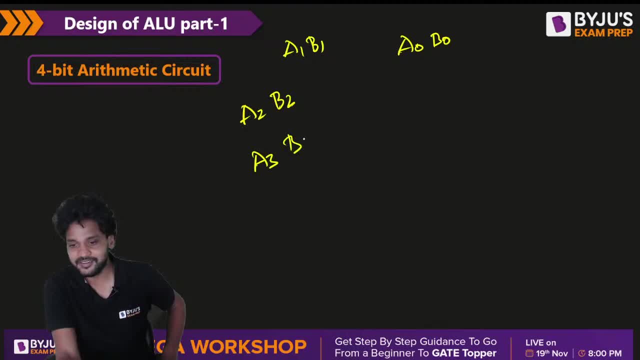 Still there is A3, B3.. Okay, So what Chinmay spotted is perfectly spot on. Due to this constraint of this recall, the space limitation, we just are able to showcase, we just are able to demonstrate or manifest only one stage of the ALU. 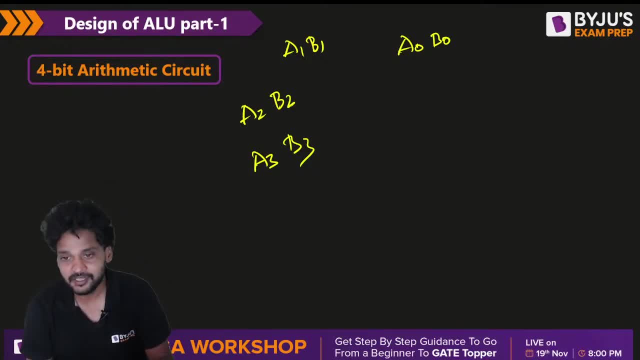 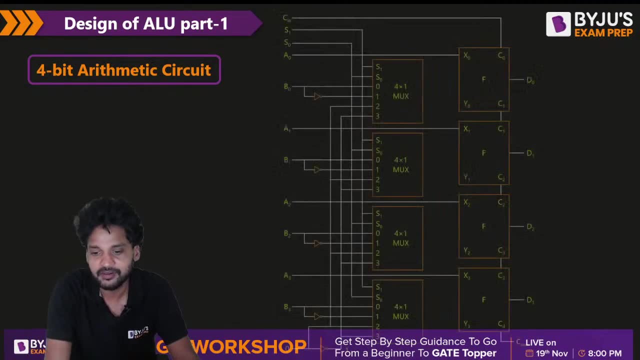 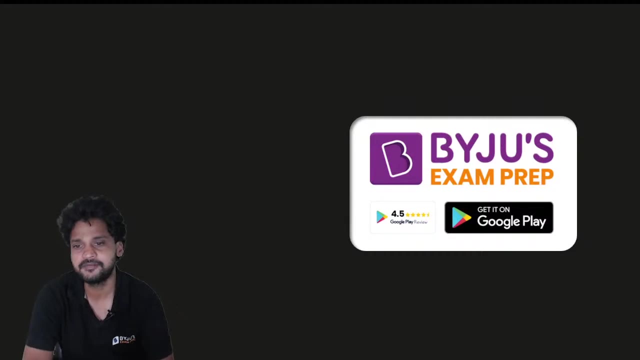 Got my point. What Chinmay told is perfectly right. So with this we have come to an end of this session. Did you get this, Chinmay? Can we sign off? Can we sign off? Please respond, Yes, Yes. 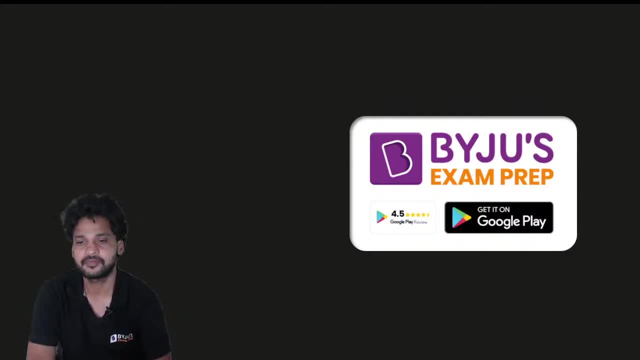 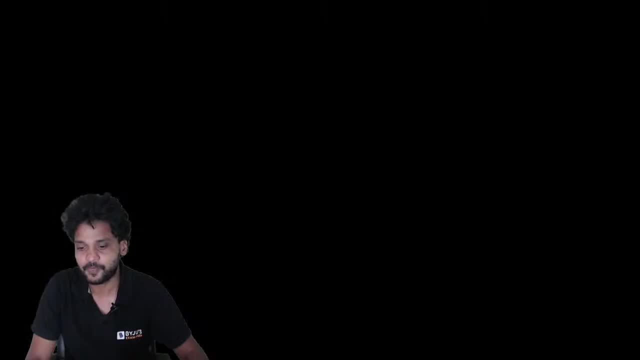 Yes, Yes, That's it for the session. Thank you so much, Anupasat Surfampudi signing off. Thank you, Anu. Thank you, Chinmay, for joining. Thank you for watching. Thank you Bye. Bye, Bye.